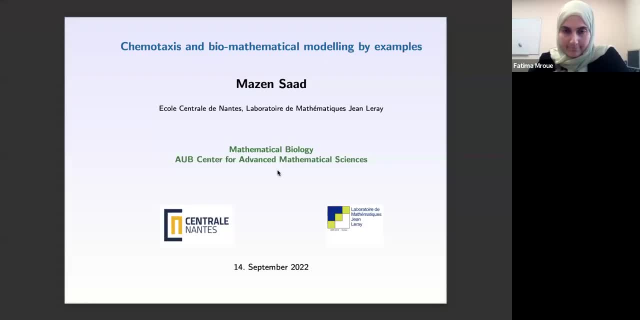 Good afternoon. Thank you for joining us in this first lecture of a series on mathematical biology. I will leave the floor to Professor Touma, the director of CAMS, to introduce the series. The floor is yours, Professor Touma. Thank you, Fatima, and thanks to Professor Saad for. 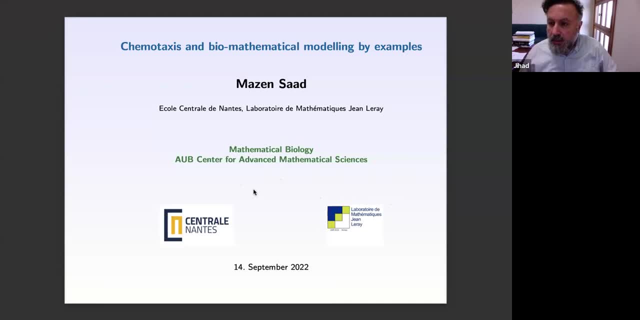 joining us for this first lecture in the series. I want to first start by thanking Dr Mrouwe for leading on this effort, practically single-handedly, to try to reflect our center's interests in mathematical biology, primarily in terms of the beauty of the field in itself. 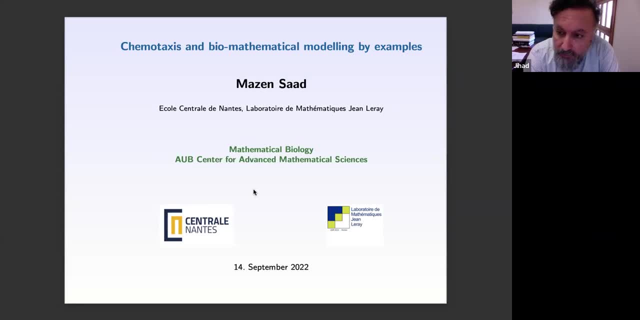 but also in terms of its implications For the context in which we're working. we're part of a university with a stellar medical school, which is also neighboring by other universities, with medical schools each involving high-level research as well as clinical practice and each benefiting potentially from the 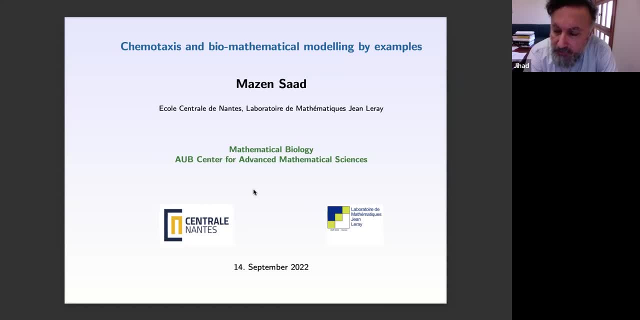 contribution of mathematics and mathematical modeling for their work. We're particularly invited in this context in terms of an initiative which we are pursuing with the medical school at AUB to catalyze and strengthen the dialogue between mathematics, mathematical modeling, data analytics, as pursued and featured through the work of CAMS and the work that is being 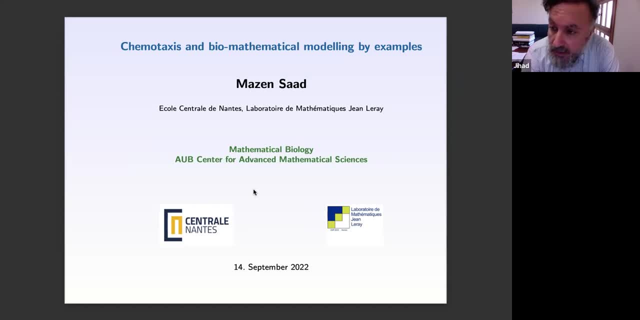 done in the medical school And, in that context, Dr Mrouwe, myself, Fatima, our colleagues in mathematics here at AUB, in biomedical engineering, with whom we've had a long-standing collaboration through CAMS, as well as our colleagues in the 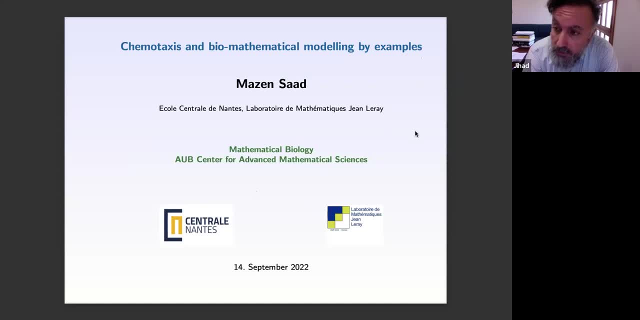 medical school are very much looking forward to the lectures as an occasion to basically start having this conversation around the issues that are of current and important importance. So, Fatima, thank you again for leading on this effort. It's been a pleasure working. 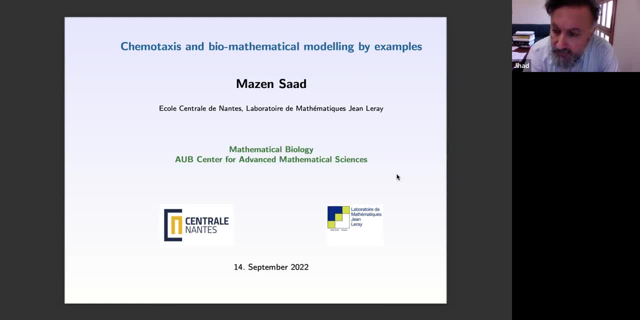 with you, and I very much look forward to what you have managed to put together for us. Thank you, Thank you. It's my pleasure to introduce Professor Mazen Saad, who's a professor of applied mathematics at the engineering school École Sainte-Haldonan, where he's 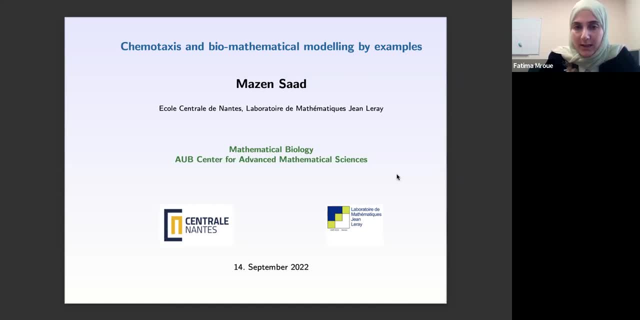 the president of the scientific council there since 2017.. He's also a professor at the University of Bordeaux. He's also a member of the Federation of mathematics, and the National French Council has attributed to Professor Saad the prime for his excellent scientific research since. 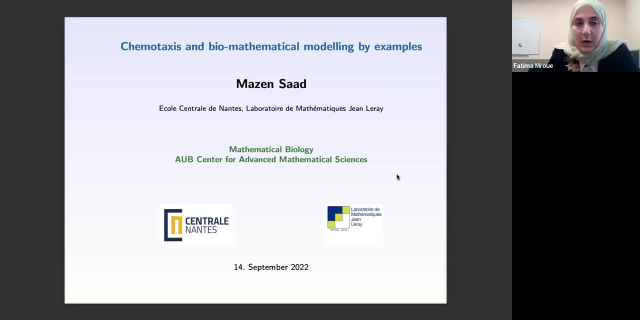 2013.. His research interests focus or are concentrated around multi-phase flow and porous media modeling in biomathematics and on finite volume methods. Thank you for being with us, Professor Saad. Goodbye, please, the floor is yours. okay, thank you, fatima. i would like to thank firstly dr fatima. 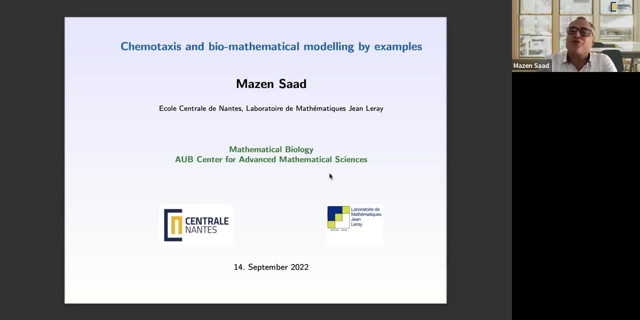 as our organizer of this talk series, fatima, asks me to, to give an overview of some of my research on biomathematical modeling, and for a large audience. i have tried to remove the technical mathematical results about existence of solution or some something like that, and i i focus my presentation on the modeling of some biological process and how to translate them. 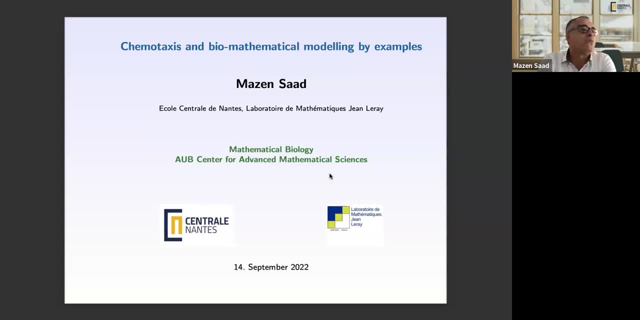 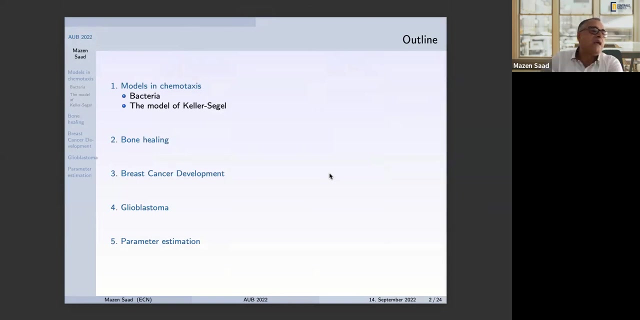 into mathematical equations and how to to solve that. you, nevertheless, i i i have to give you in my presentation some equations or operator modeling, biological. for the outline of my presentation, i'll introduce the process of chemotaxis and i'll give you some examples to illustrate. 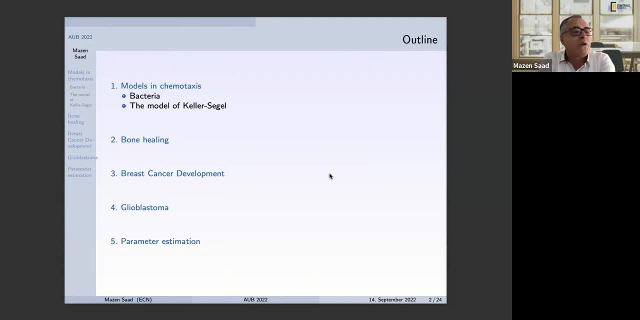 the process, especially, especially, the model of the rest of my talk. in is a succession of examples. okay, i give you here for each. for each example, i will specify the biological pro process and the mathematical model, and some numerical results will will be presented. the first example concerns bone healing. the second one is about the breast cancer initiation. 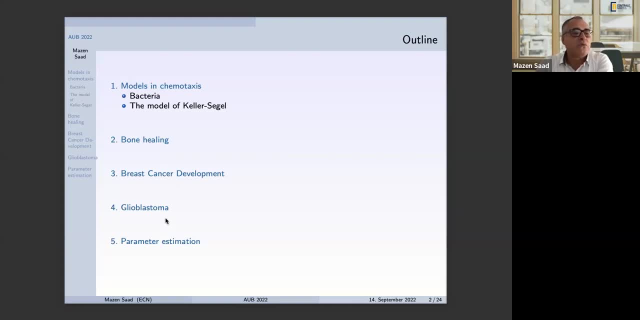 and the third one here aims to understand the brain cancer, the glioblastoma and finally, in the context of personalized medicine, how to calibrate the biological parameters with the help of data as MRI and some analysis of passion. Okay, let us first define what is chemotaxis. 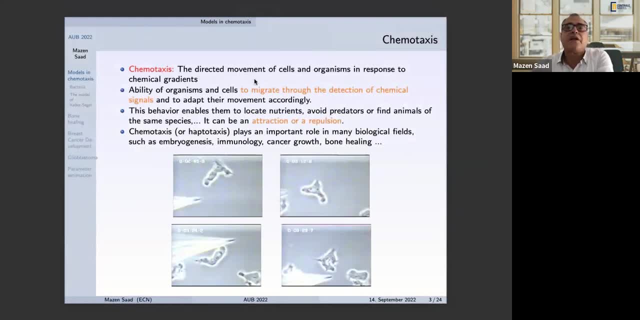 Chemotaxis can be defined as directed movement of cells and the organism in response to a chemical signal or a chemical gradient. Chemotaxis is the ability of organisms and cells to immigrate through the detection of chemical signals and to adapt their movement accordingly. This behavior of cells enables them to locate nutrients, avoid predators. 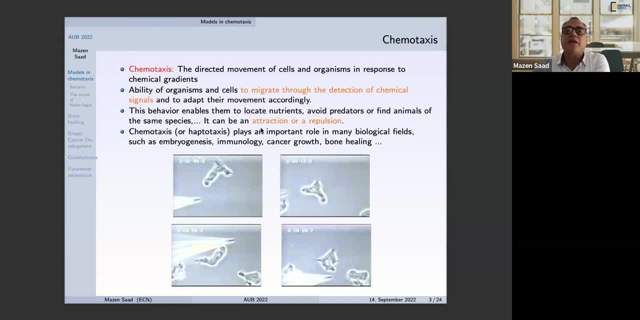 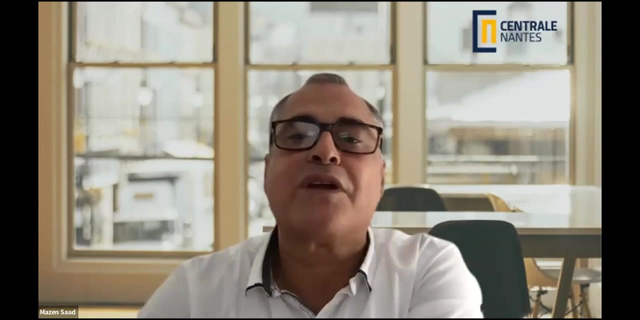 and prevent disease. Chemotaxis is the ability of organisms and cells to immigrate through the detection of chemical signals and to adapt their movement accordingly, and it can be an attraction or repetition. I show you here, only in this, my talk, one video. so I have to stop share here, sorry. 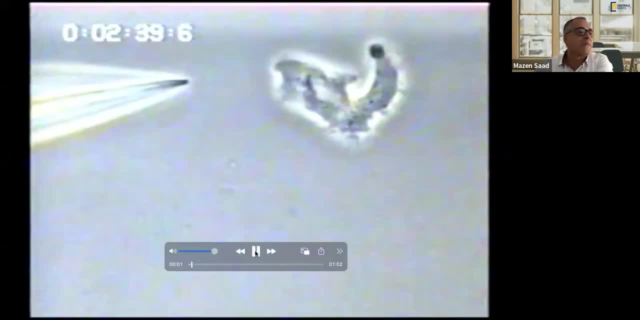 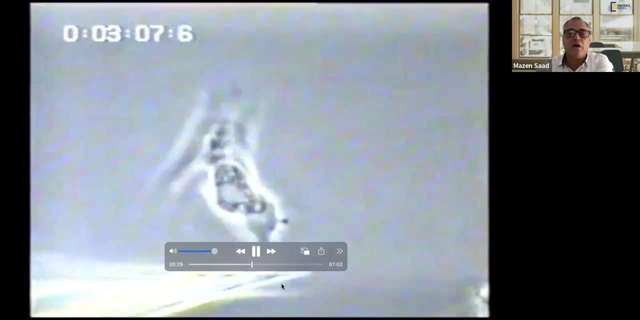 okay to illustrate this mechanism. We can see in this video that is here a pipette swapped by a chemical specie and here this organism, or multicellular organism, detects the chemical and then it modifies its displacement according to, here, the high concentration of the chemical. And we see here also another organism who are attracted by this signal. 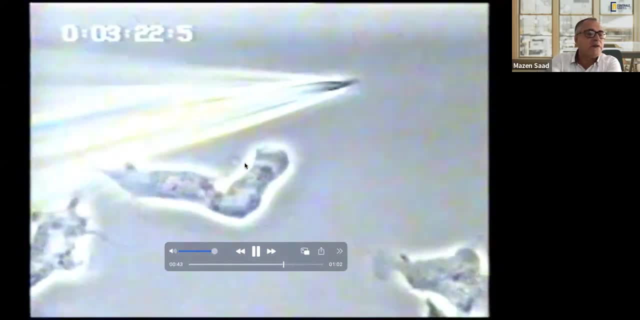 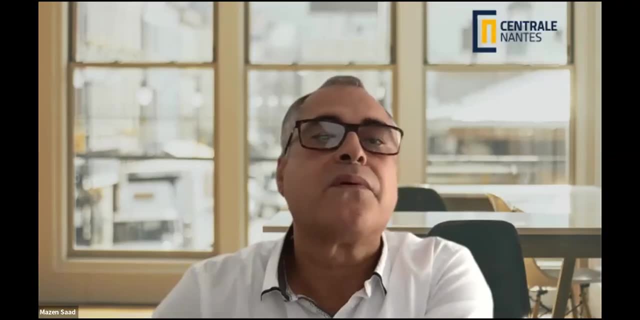 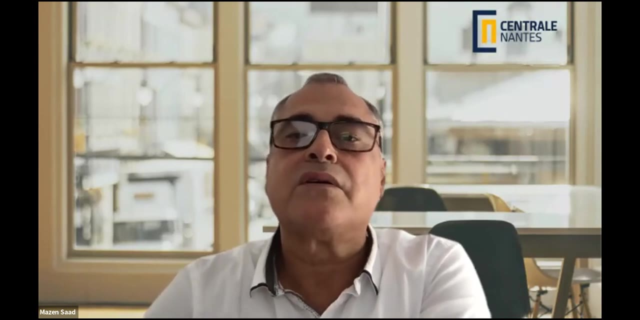 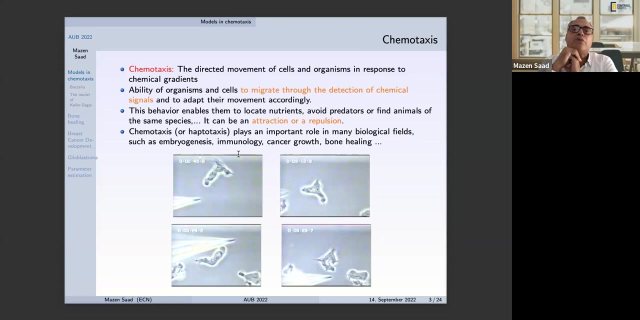 Chemotaxis is a vital characterisation of living organism to adapt their movement. Okay, And I switch to and, and Chemotaxis, or we say also haptotaxis. haptotaxis is where the signal is not in full width, perhaps as enzymes. 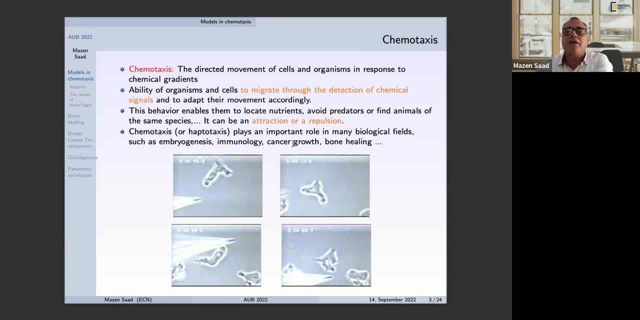 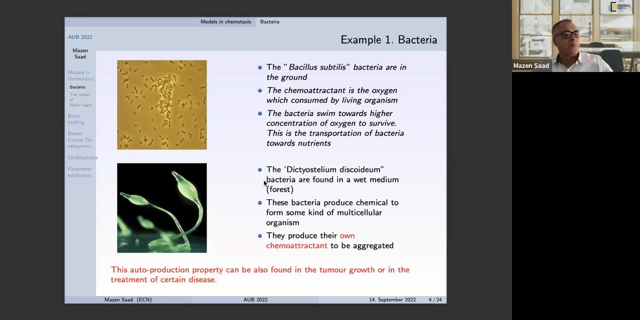 we say here about haptotaxis. They play an important role in many biological fields, and especially here. what we say is a gross cancer, the bone healing, et cetera. The first example here is given by the bacteria Bacillus septuulus. 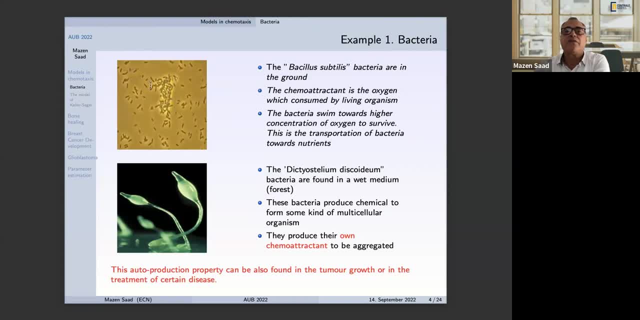 This bacteria can be found in the ground. The bacteria here move towards high concentration in oxygen here to survive. The nutrient here or the chemoactivant are the excision And chemotaxis is also can be view as a transportation of bacteria towards the nutrient. 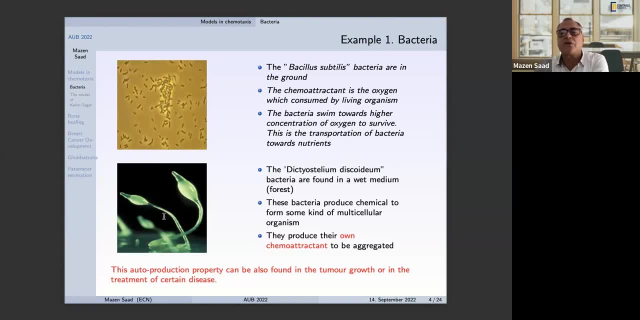 Another example here is the DDC bacteria, which we can found here in a wet medium In the absence of nutrient. a specific characterization of this bacteria is the production by themselves of chemical to be aggregate, And this autoproduction property can be found. 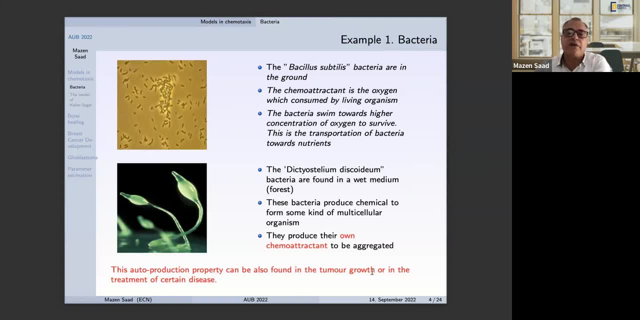 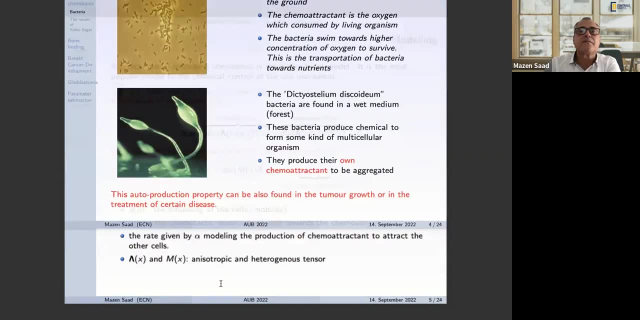 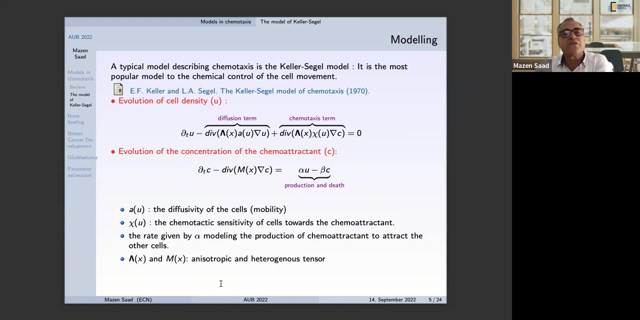 in the tumor growth and play very a major role in the tumor growth or in the treatment in certain results. Biomathematical modeling is based on the combination, the combination- combination okay- Of three phenomena: diffusion, transport and reaction. 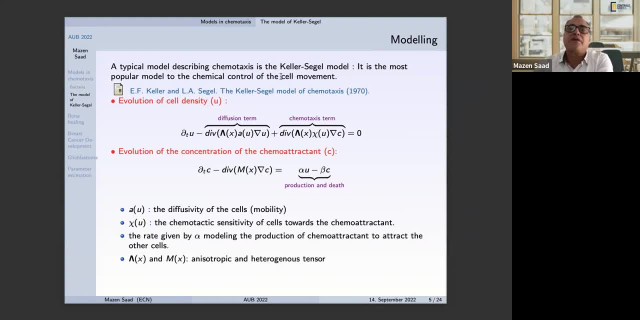 And the typical model describing chemotaxy is a killer-siegel model. It is very the most popular model to the chemical control of cell movement. The killer-siegel system is a model of population dynamics describing the equation of cell movement. The killer-siegel system is a model of population dynamics describing the equation of cell movement. 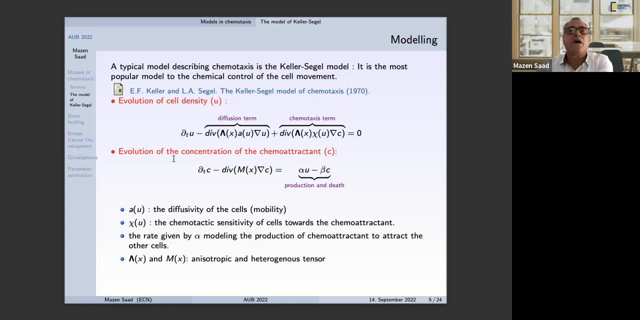 The killer-siegel system is a model of population dynamics describing the equation of cell movement, The evolution of the cell density and the evolution of the concentration of the chemoattractant. The cell density equation in here contains two terms. The first one modeling the diffusivity process. 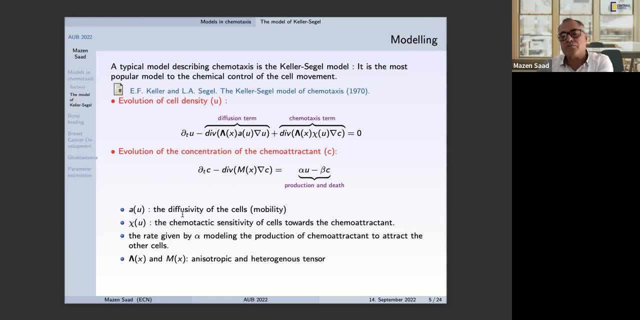 And here A is the mobility or the function of diffusivity of the cell, of the cells, And next is the concentration. The second term represents the chemotaxis term. This term represents the response of cells to the gradient of a high concentration given by the gradient of C. 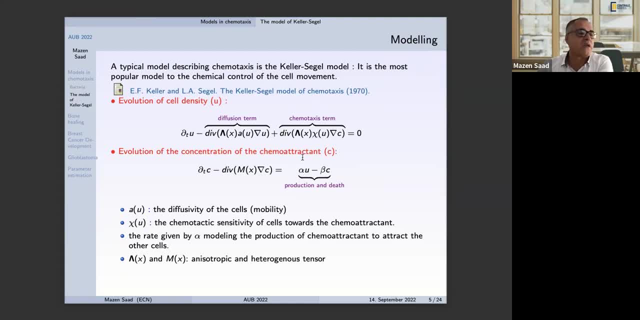 and C is the concentration of chemoattractants. This operator, we can see it as a transport operator. It means here that Chi is the chemotactic sensitivity of cells, and the cells are attracted or are directed according to a velocity. 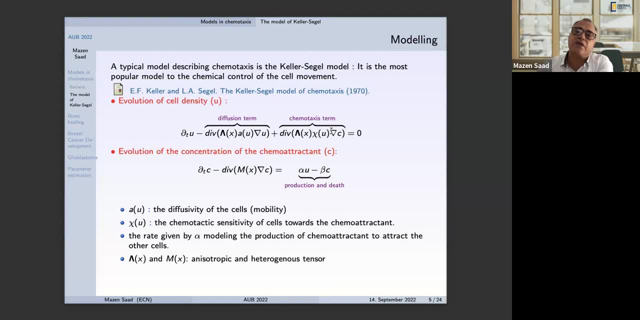 and the velocity here is minus the gradient of C. It's a transport equation and the cells detect this signal and it is directed to the high concentration of chemoattractants. Here we have the sine plus, It is the attraction. 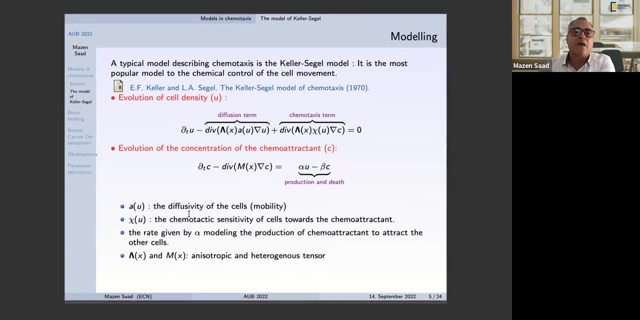 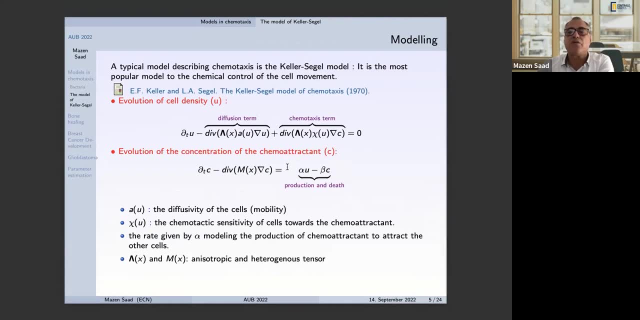 If you take here minus, it's a repulsion phenomenon. Next, for the concentration of the chemoattractant. here we have a simple diffusion equation. We have only a diffusion term here. and to model the production of chemoattractants, 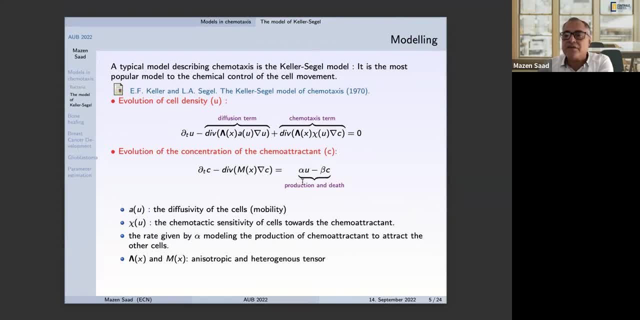 it is modeled here in this term The rate given here by alpha modeling, the production of chemoattractants to attract the other cells, And here beta is the rate of death of the chemoattractant. We can add in this model two tonsors. 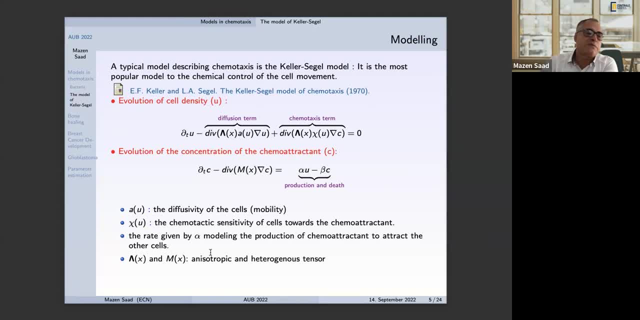 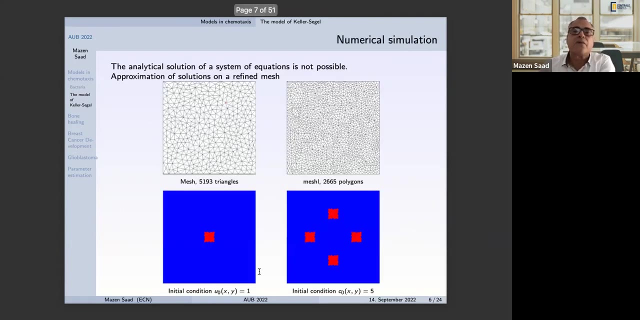 lambda and n to specify: is the medium where the film is a cure, is isopropic or non-isotropic or heterogeneous? Okay, We are interested mainly in the numerical approximation or numerical resolution of this kind of equations. Just in a few words. 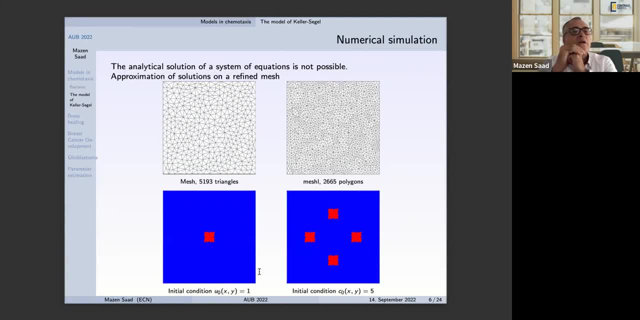 in mathematics in general, we are not able to calculate the exact or the analytic solution of a system of nonlinear or linear system. Okay, It is only for academic equation. we can compute the solution, It's okay. But in general, for the real problem, 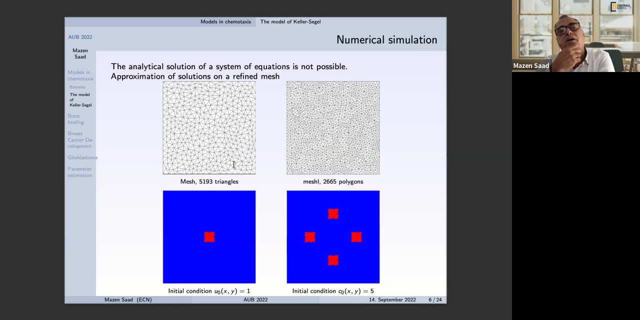 it's not possible to exhibit exact solution For that. we construct numerical methods to approximate the solution on measures as fine as we want, And next we calculate the approximation of the solution on this mesh. For example, if you take this mesh with: 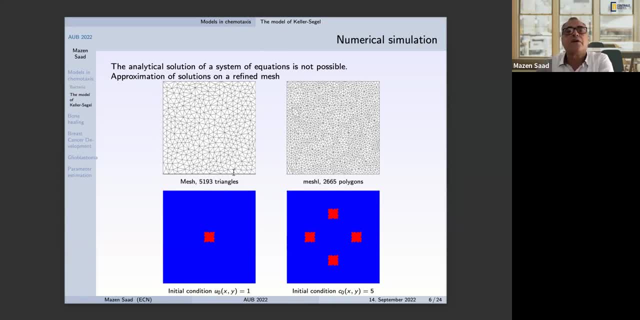 for example, 500 triangles. it means that we are able to give an approximation of the solution at 5,000 points in this domain and which give a very good approximation of the solution. Okay, And we compute at the center of the triangle. 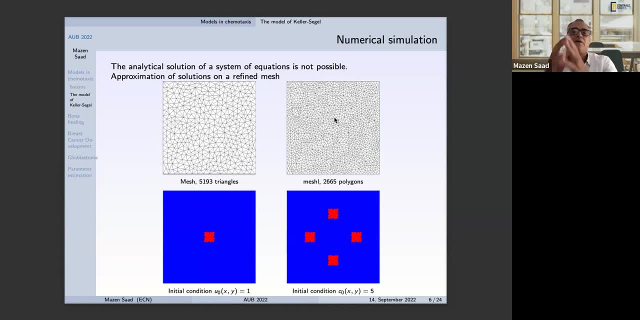 or the center of the vertex of any polygons, et cetera. It's a big, big, very large domain in applied mathematics: how to construct a numerical scheme and how to solve this equation. Okay, To show the behavior here of the solution of the killer signal. 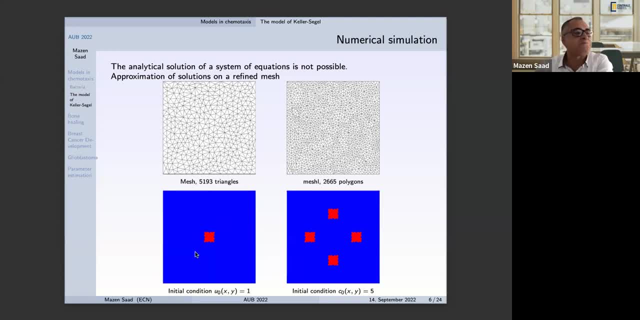 we simulate here the evolution of cell density starting from uh, the initial density, which equal equal one in the red square here in the center, And uh and the chemoattractant are located here, uh, around. 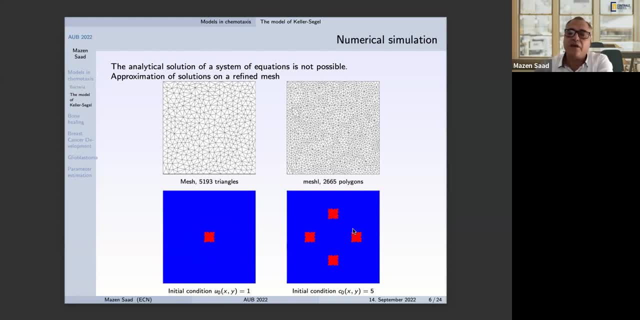 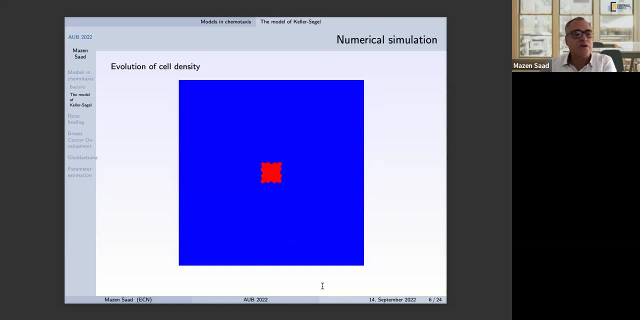 uh the cell density, uh in, uh the pore spot here. Okay, We start from the initial uh uh, first the we have the density of cells. evolve uh by diffusion, uh since the deep. 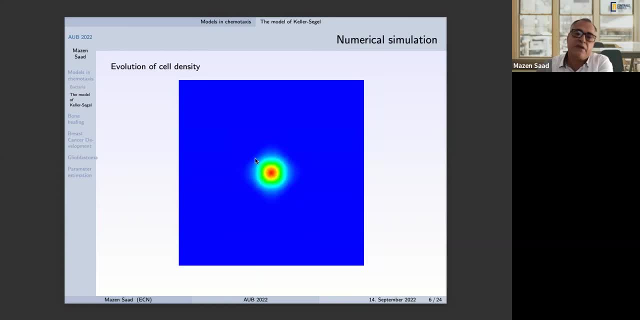 this: if you look here, this placement: uh, it is symmetric and uniform in all direction. This is a random distribution. Uh, it means here the diffusion, uh, contribution is. uh is important. uh is the first stage in the evolution. 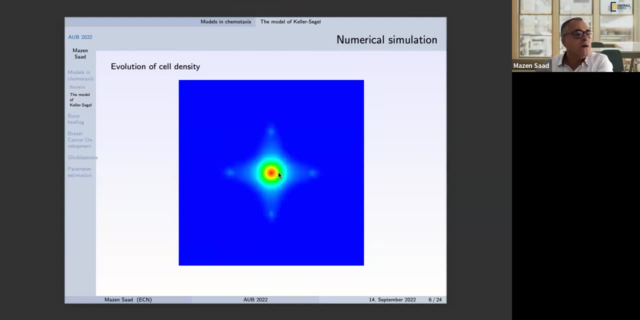 uh of the system And next, after a short time, the cells detect the chemoattractant here, which are placed around the density center in this one, And here we see the influence of the chemotaxis operator and the transport of cells to the 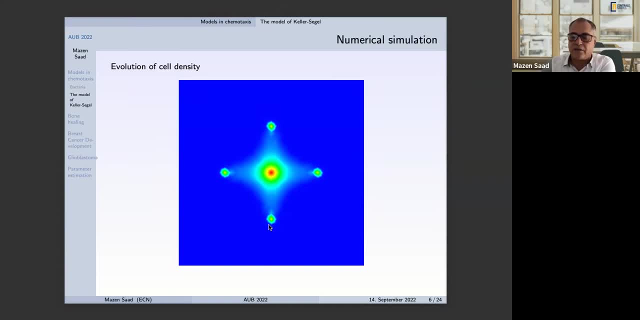 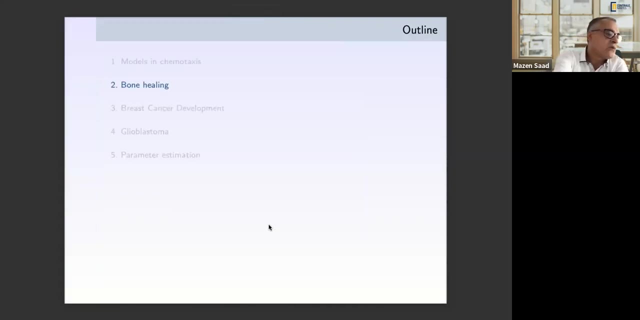 site here of chemoattractant, And the attraction continues, okay, when the time increases. Okay, this is the main phenomena for the killer signal system. Okay, and now. the first example where chemotaxis play a major role Is bone regeneration. 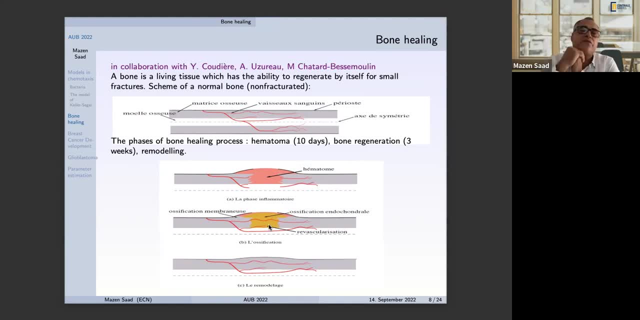 We begin by before writing the equations or the model in mathematics. firstly, we have to understand what is the biological process And we begin by describing the biological process. This work is in collaboration with Yves Caudillard and Ysereau. 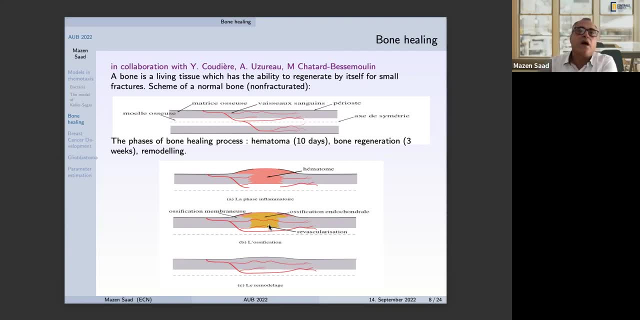 A bone is a living tissue which has the ability to regenerate by itself for small fracture After a fracture. the three steps of bone healing process are: firstly, we have a hematoma step during 10 days. this is the first stage And the seventh step is the bone regeneration. 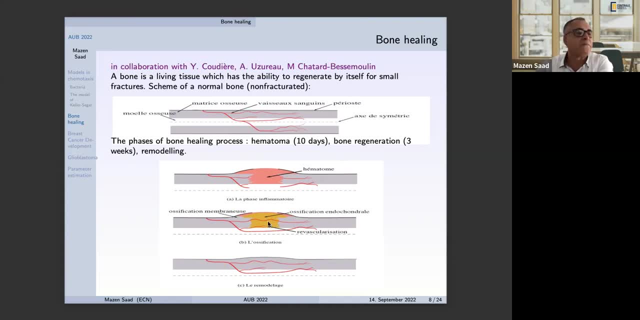 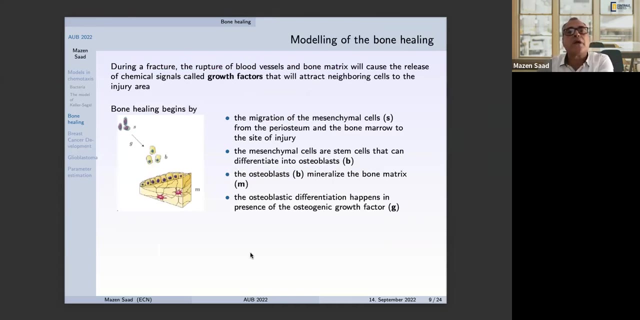 It is a ossification of the membrane during three weeks, And the last step is remodeling of the bone. During a fracture, the rupture of blood vessels and bone matrix will cause the hematoma to be reduced. Okay, And then we have the release of chemical signals called the growth factor. 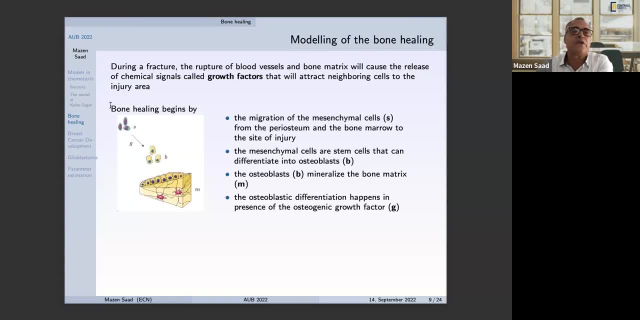 And that will attract neighboring cell to the engineering area. In this scheme I show you the mechanism of the bone healing. The bone healing begins by, firstly, by the migration of these unchemical cells. They are the stem cells, And these stem cells are present in the period of the bone. 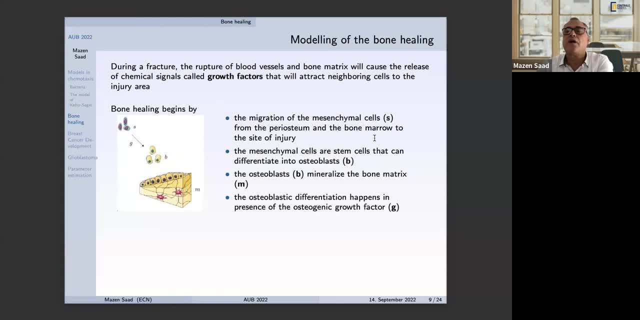 in the periosteum and the bone marrow and this stem cells immigrate to the site of the engine. And next, stem cells here in the presence this factor- growth factor- differentiate into osteoblasts. And next, this osteoblasts mineralize the bone matrix. 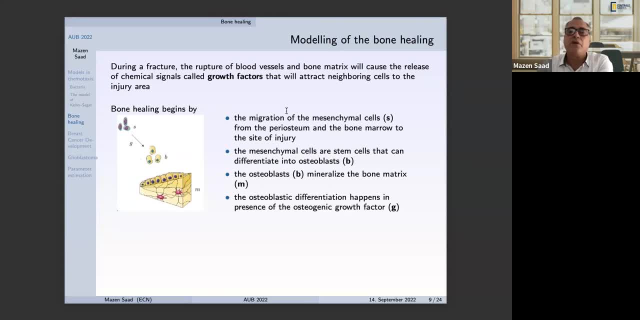 to construct the bone. And all this phenomena can be occur, or can be happen when in the presence of osteogenic growth factor, and it is a chemoattractant in our analysis. Okay, now we want to translate this, this biological process, in mathematical equations. 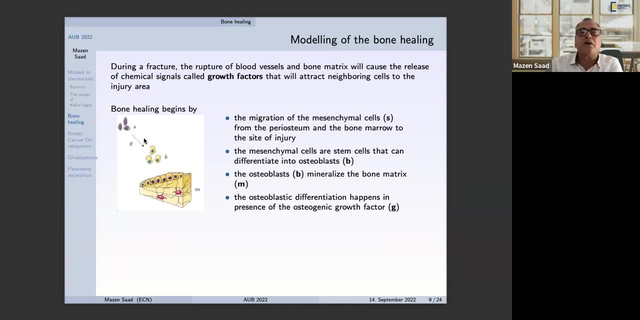 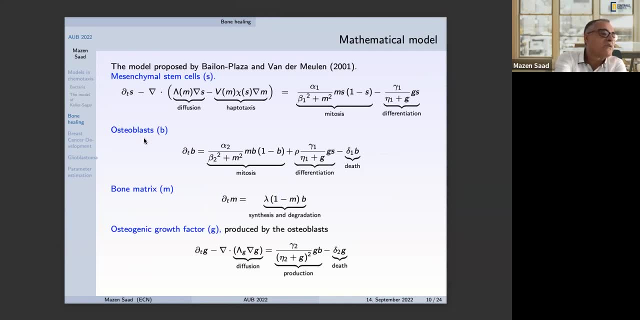 to try to solve the bone healing. Here we consider the model proposed by Bailan-Plaza and Wadern-Nuland, which take here into account the several mechanism of the bone regeneration process. For the stem cells we find here the killer signal operator. 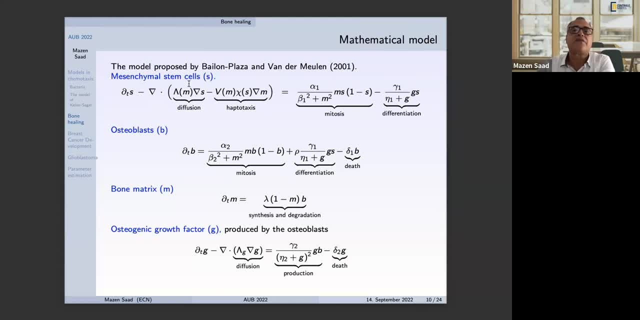 Firstly, we have the diffusion operator of the stem cells And the second one is the haptotaxis term, And the haptotaxis term here is due to the presence of the high concentration of the haptotaxis in the bone matrix- is two gradient of M. 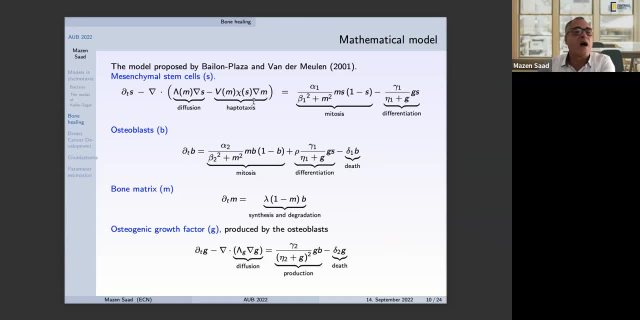 So here the stem cells are directed towards the region where the variation of the bone matrix is high- and here is the bone matrix and which exactly the injury is on- or for example, where we have a factor okay And we have here the reaction term. 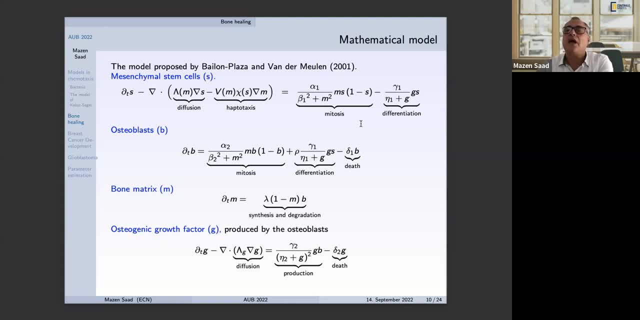 We have firstly the methylosis and we find here the differentiation of stem cells to be transformed. in this term is transformed in osteoblast here, And rho- here is the quotient of conversion, or from stem cells to osteoblast. 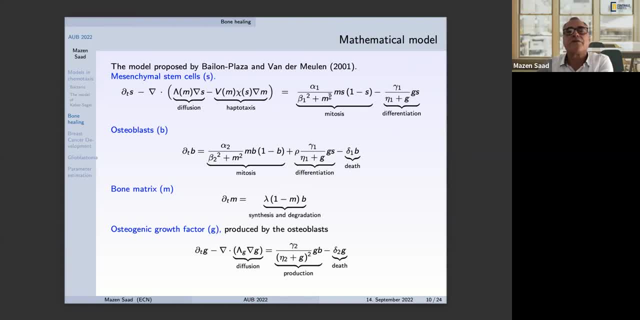 Okay, this term here is negative. That means stem cells are here transforming on osteoblast. This is the differentiation process And in this mechanism, all because it's biological- we need to have the growth factor here, G, to ensure that the reaction happens. 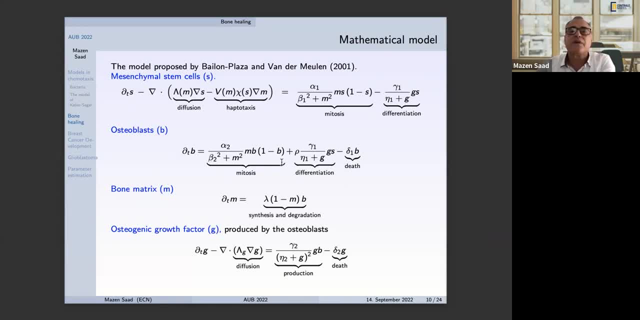 The osteoblasts here are fixed on the bone Because there is no evolution term. It is a simple ODE equation: And the bone matrix here we have. we have the bone matrix here, and the bone matrix here we have. 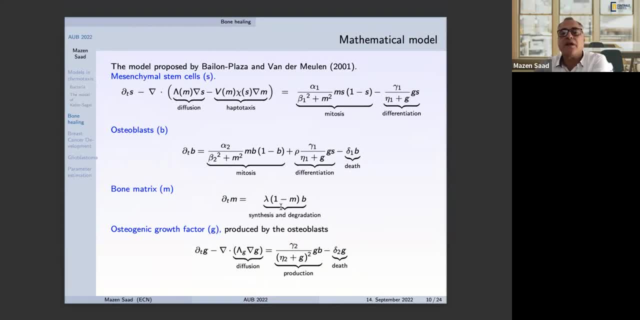 we have the transformation of the osteoblast in bone, which is the term lambda B, And we have also the degradation of the bone, by the term minus B. The osteoblast degrade- degrade also as a bone matrix, Okay, and finally we have here the osteogenic growth factor. 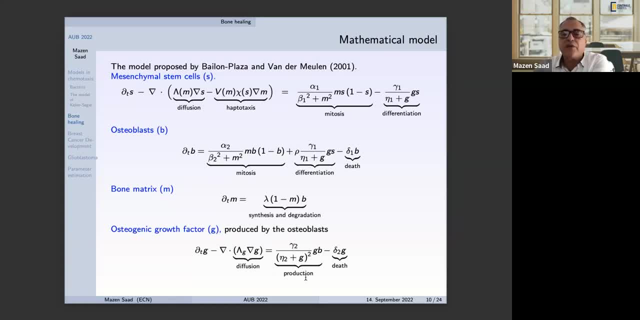 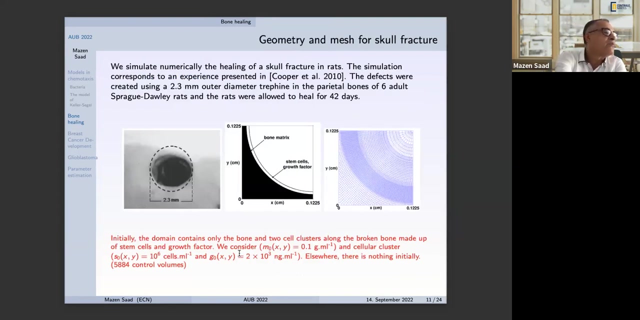 which is produced by osteoblast. Here we have the production of growth factor by the presence of the osteoblast. It is the auto-production, okay, of growth factor, The due, due term to increase the healing of the bone. Okay, I give you, only here, numerical simulation. 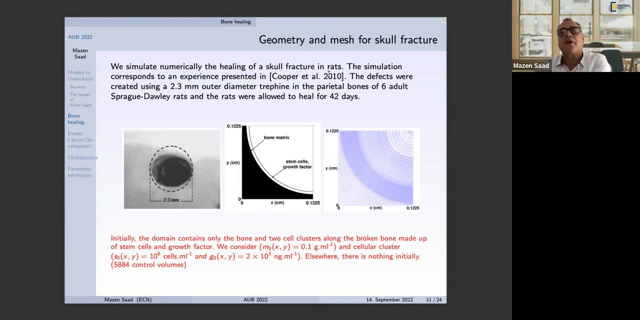 We simulate here in the healing of scar fracture in raties. This simulation correspond to an experience presented in the paper of Cooper, and all And here is an effect is a whole fracture with a 2.3 millimeters Okay, and we consider here the whole fracture is symmetric, for that we simulate only the quarter of the domain. 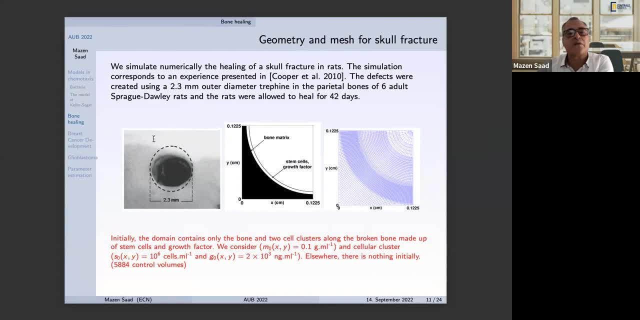 Okay, we take the quarter is. this part is a quarter here and the dark region here is a bone and the white region is a fracture. Okay, The domain here contain only the bone and we place here the two cluster along the broken bone. The broken bone here is the friend between the dark and white region. 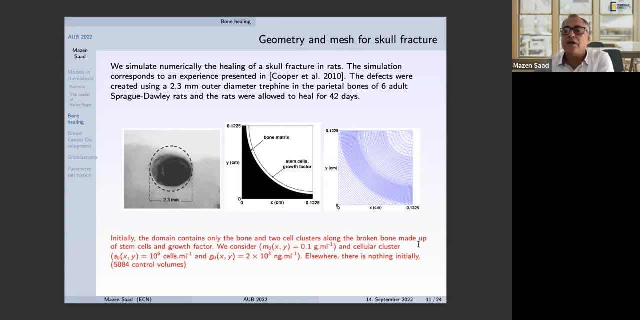 The fracture and the And the. initially we have only stem cells and the growth factor. Okay, and we are blessed. near the fractal here, only between the dark region and the perfect line. this one Is a simulation of the scale. factor needs Is a construction of complex mesh and 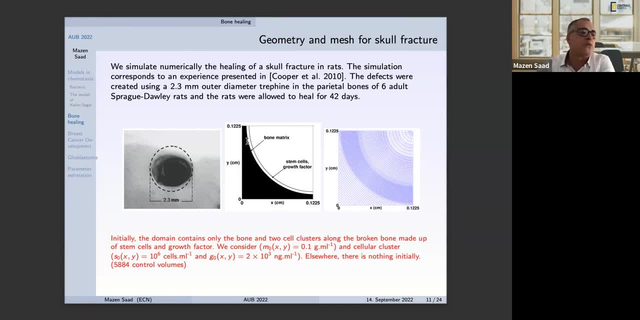 Is a mesh is refined. refined here around the injury region, Because all biological phenomena are happens here in this region and we want to to, We are evil to, To consider an accurate. we need. we need an accurate solution near this region. okay, For that we consider refined mesh about in this one. 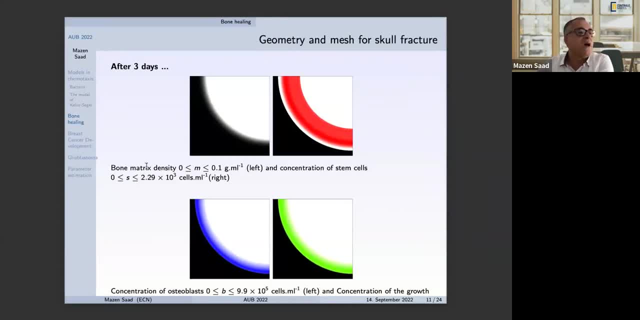 Okay, we see here the bone healing after three days. after three day, we observe, firstly, the formation of osteoblasts, Because it's a blast- are not initially present, You have the creation of the osteoblast, And This also plus. 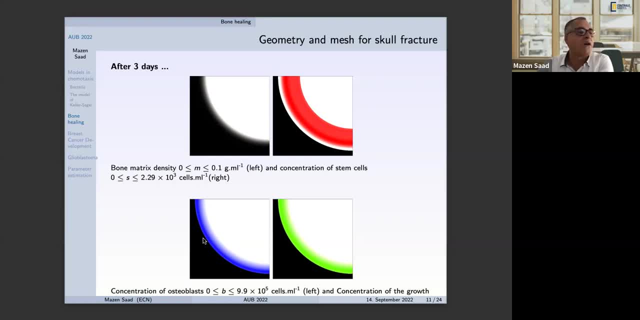 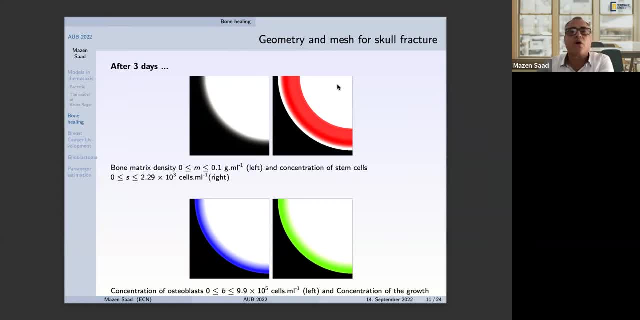 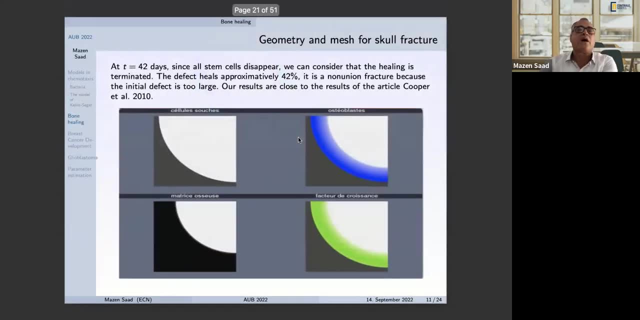 Are Move Towards the Center Of the. Okay, after 42 days, Here as a stem cells disappear And it is here in this, in this year, And We, in this case, we can, can, we can consider that the healing. 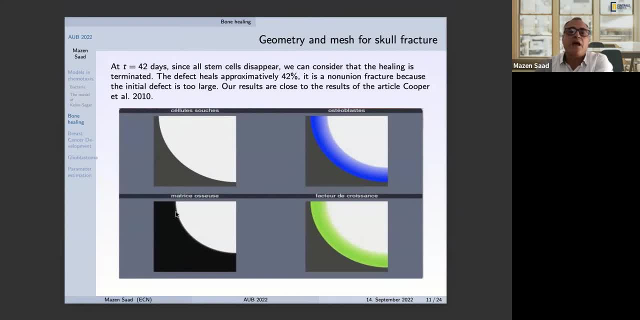 Is is actually okay And we have. here is the final Formation of the bone in in it's a given in this figure. Okay, and here we calculate. that is a defect. healing is approximately 42% And here we see that there is no union factor. 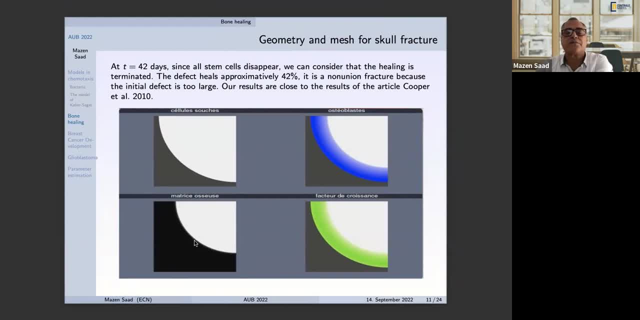 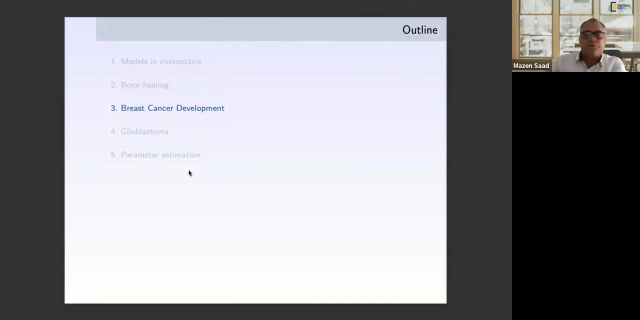 Because the initial defect is is too long. Okay, and we, here we are. we find that our results are very close to the article of Cooper. to validate Some of the model and the numerical Approximation. Okay, now in the next part, 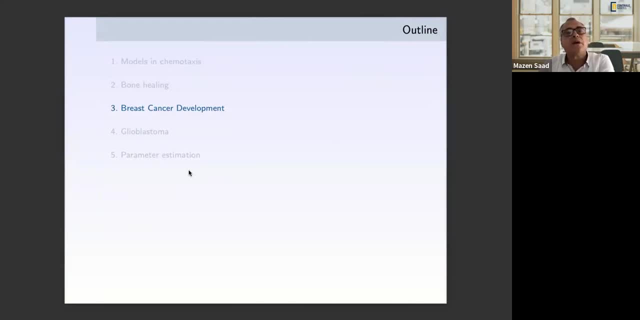 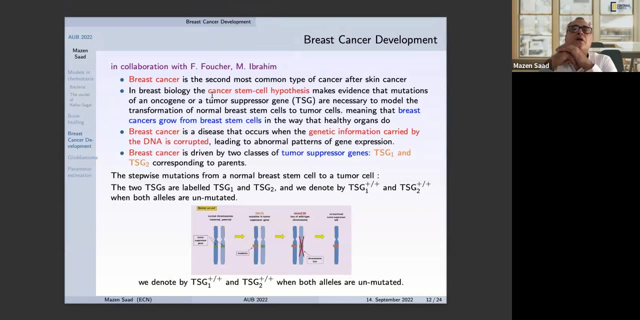 We focus in a breast cancer Initiation. This work is a is in collaboration with the process to share and most of it Brass. breast cancer is the second most Type of cancer after skin cancer. Okay, We are interested here in the initiation of the breast cancer by modeling the step, the stepwise mutation from a breast cell, normal breast cell or head to the cell. 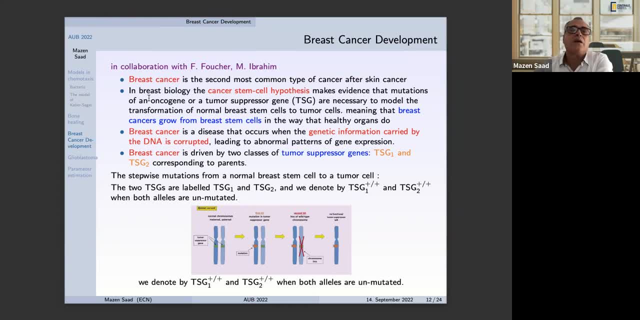 To a tumor cell In breast biobiology the cancer stem cells I put. I put is Makes evidence that mutation of an oncogen or tumor suppressor gene, TIG, are near necessary to model That transformation, or of normal person to tumors. 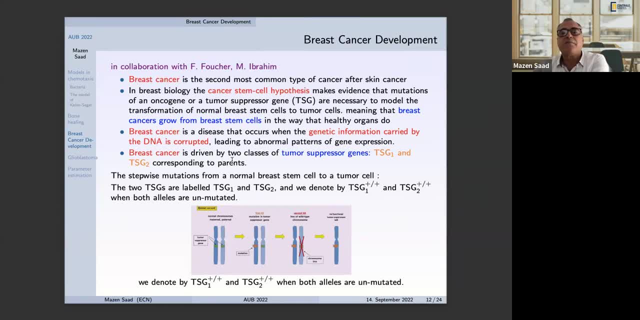 And breast cancer. here is driving by two classes of oncogen. In the second class, Or tumor suppressive gene, We denote here by TIG, Jee won, enteage of it, and which correspond to parents. Is that to TIG here? or maybe the TIG one and TIG two? 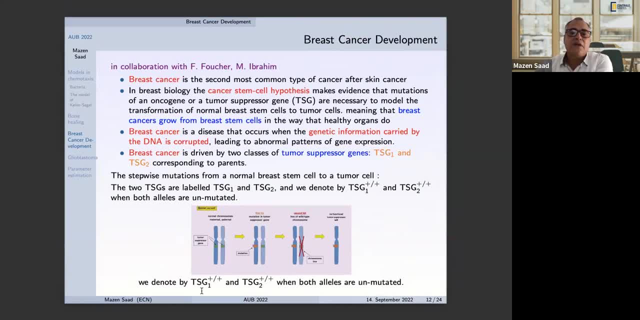 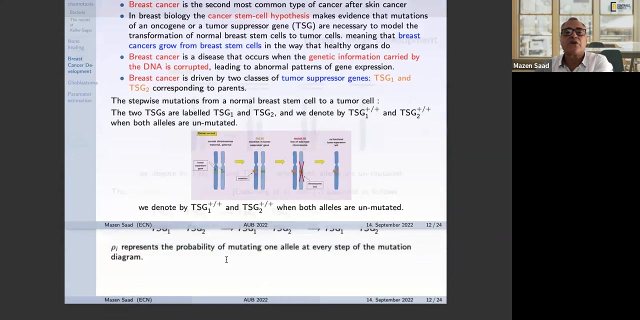 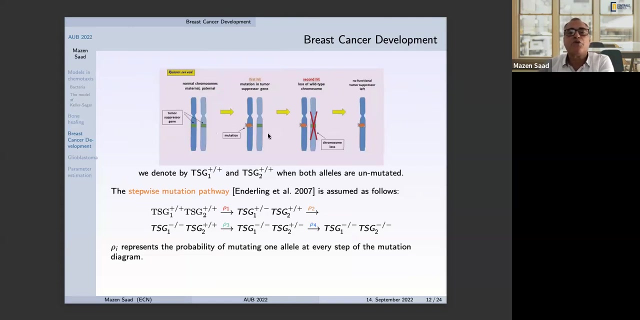 And next We denote by I TIG one plus plus and TIG two plus plus, And as a oncogene, where the two alleles are not mutated. Okay, another term we can write here. I'll show you. We describe here the mutation, the step mutation pathway. 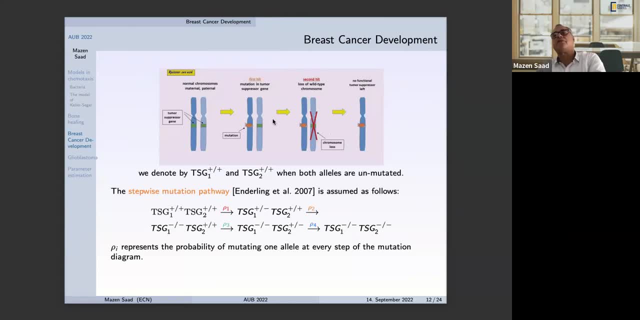 to explain the initiation of the mutation Of the breast cancer. We consider here the mutation diagram given in the paper of Enderling And we consider this diagram of mutation. We denote: firstly, we consider rho i. here is the probability of mutation. 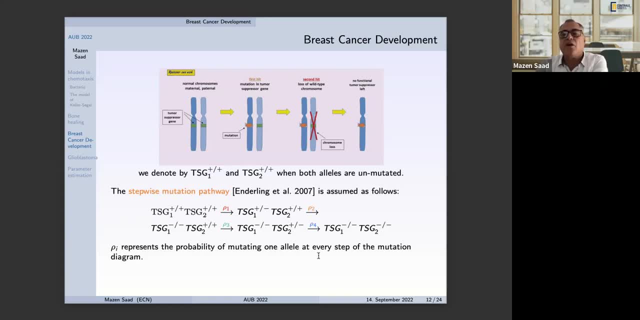 of mutating one allele of every step of the mutation in this mutation diagram here, And we consider this implication of the mutation. If you consider here, rho i, rho i is the probability of mutating one allele of TSG1, okay, Rho i and next after this step. now we pass the second step. 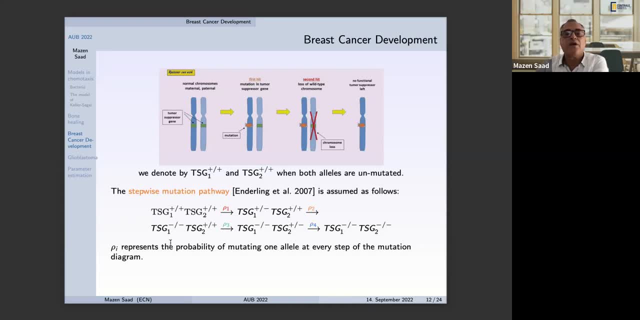 step is the root 2, and root 2 is the probability to SG1 of muting of the second LED. okay, And we consider now the SG1 is completely muted And next we pass now to SG2, and to SG2. here we have the probability for SG2 of muting of one LED. Now we have plus minus. 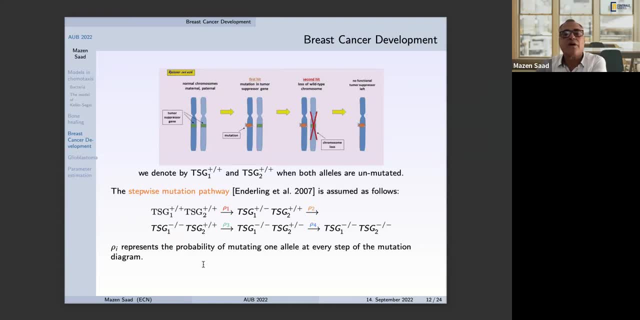 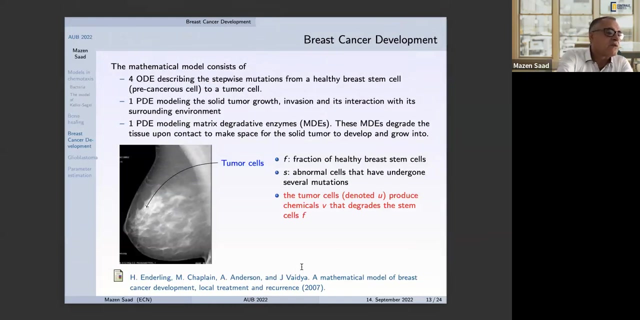 and finally, row 4 is the probability okay, for the two SG are now completely muted And we consider this cell is now. is the constitution To model this, to translate this, okay, this diagram in equations we consider firstly four: ODE is our. 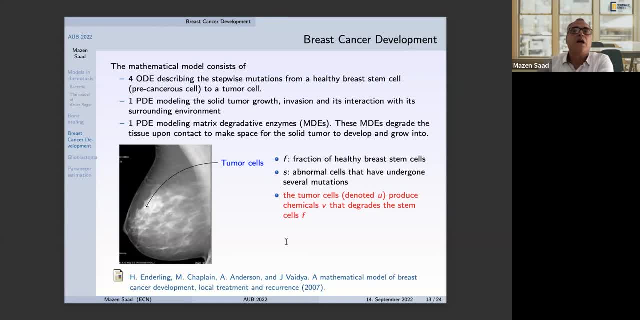 differential, ordinary differential equation here describing the stepwise mutation from the healthy breast cell to a tumor cell. When tumor cells are here, we consider now one PDE partial differential equation. we consider here the evolution of the tumor by considering a killer signal type system. We have one PDE equation to model the solid. 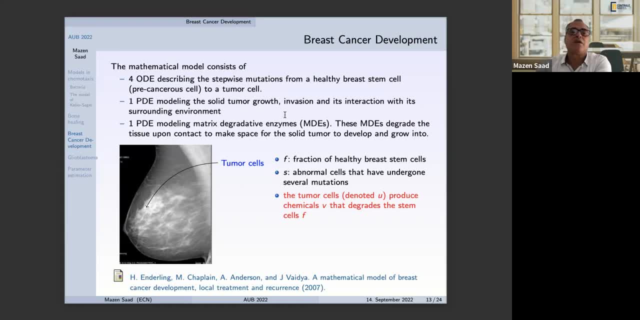 tumor growth and it is invasion in the breast. And we have also one partial differential equation modeling here the matrix degradative of enzymes we denote here NDE, and this NDE degrades the tissue upon contact to make space for the solid tumor to develop and grow into. okay, 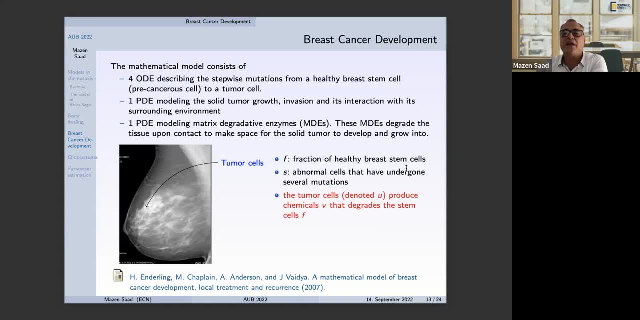 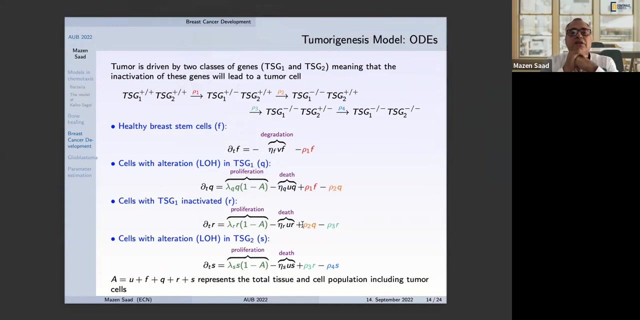 we denote here, f, the fraction of the healthy breast cell, and we denote y, u is the tumor cell and the produced by chemical, here the enzymes v, which degrade the stem cells. okay, to explain the mechanism. and now we write the equation for that. we write the equilibrium equation for each cell. 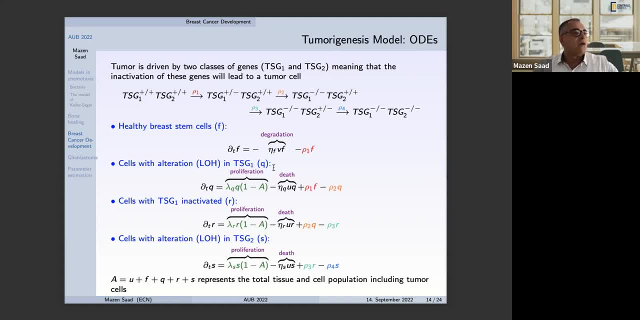 okay, we translate now, okay, the in terms of reaction equation or balanced equation, the genetic mutation for: for this system, firstly, we denote here I give you the notation: the inactivation is skipping to the callkok- hani letter of 0.a of a gene requires two alterations. 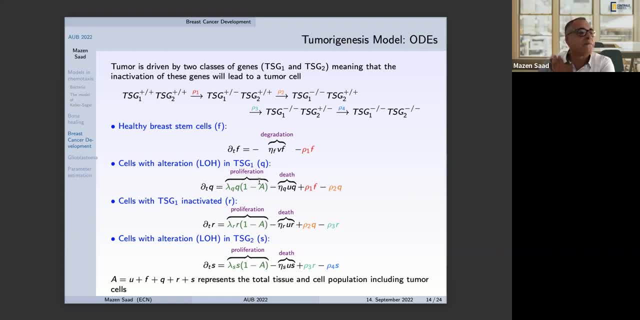 For that we denote by Q here a cell alteration. or we talk about L-O-H in T-SG1, okay, And we denote here by Q, And next we denote by R as a cell T-SG1, completely inactivate. 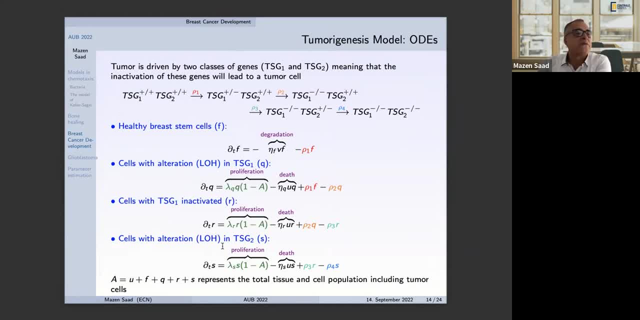 And next we denote by S, as a cell alteration, L-O-H in the T-SG2.. Okay, for the first equation. it is the fraction of the healthy breast stem cells. We write here a balanced equation. We write the evolution of this fraction. 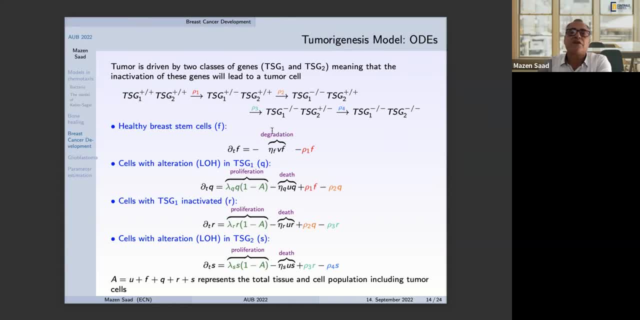 Firstly, you have the degradation- The degradation of healthy cell here is due- of V, and V represents the concentration of enzymes. okay, Then healthy cells degraded in the presence of the enzymes. And here we have the degradation of healthy cells. And here we see here exactly the alteration. 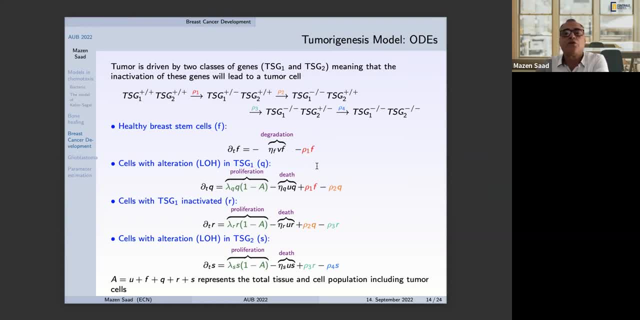 of this healthy cell by the probability Rho1 to be the first class of cells with alteration in T-SG1. This quantity is exactly the same as this one, And now we have a diagram, a diagram here to pass from cells to another, from mutation to another. 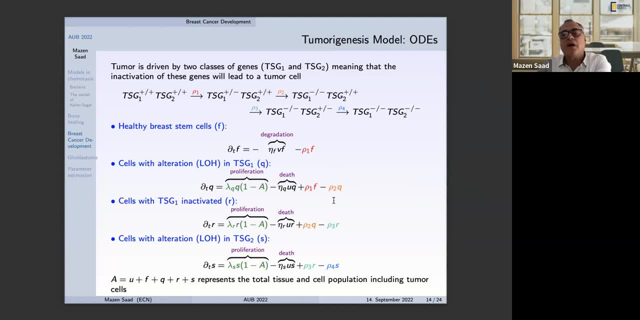 And now T-SG1. here, when the second LLE is mutated, you have minus Rho2, with probability Rho2, and we find this term in exactly in the term in R, And we continue for this class, T-SG1, Rho2.. 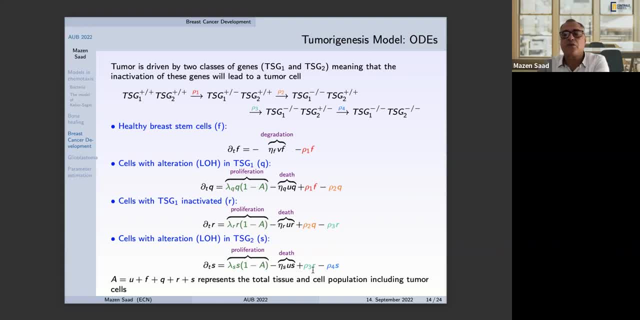 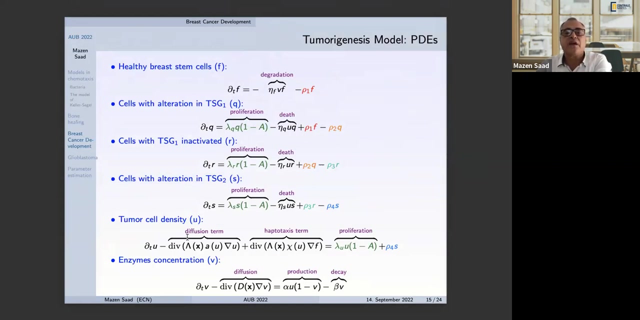 Minus, minus, And next we obtain Rho2 and Rho4. And finally, after this transformation, when the mutation is complete, now we add here the tumor cell density and we consider the cell is now is cancerous. 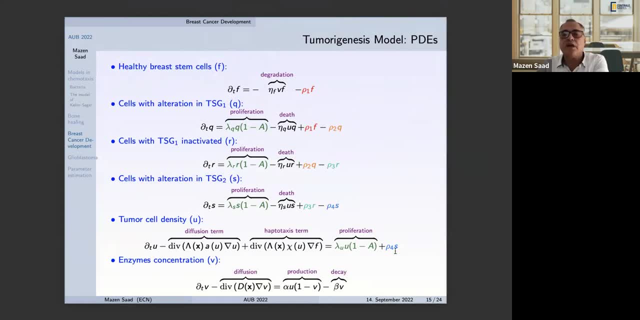 and we add this Rho2.. And this is the contribution in the tumor cell evolution. Okay, for the tumor cell density, the evolution we consider here is the same as is the same for you now, as the clear cycle model We have here the diffusion of the tumor cell. 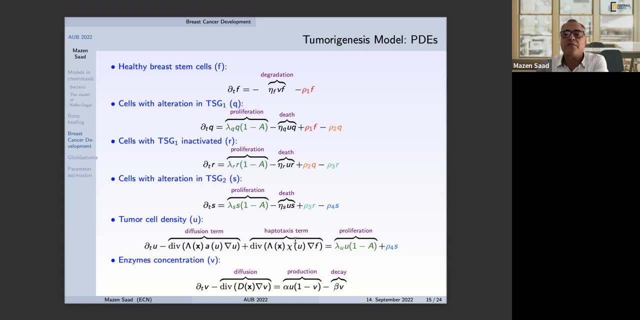 and we have here the up to Texas term, and this term is directed by the high, the gradient of the healthy, the healthy cell. Okay, the tumor gradient is directed to the high gradient of the healthy cell. Okay, and we add here the proliferation terms. 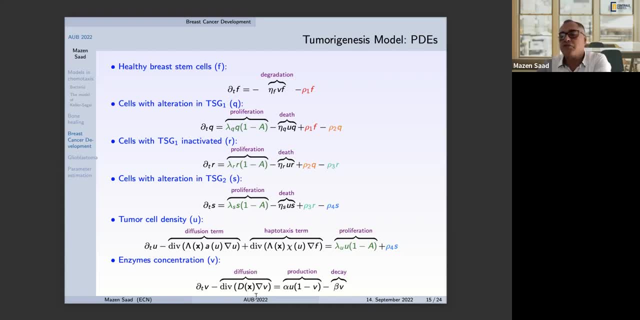 For the enzyme concentration we have simply a diffusion term and we add here the production of enzymes in the presence of density, because here we have the plus alpha U and the U, here is the density of the tumor cells And we have also is a decay indicator. 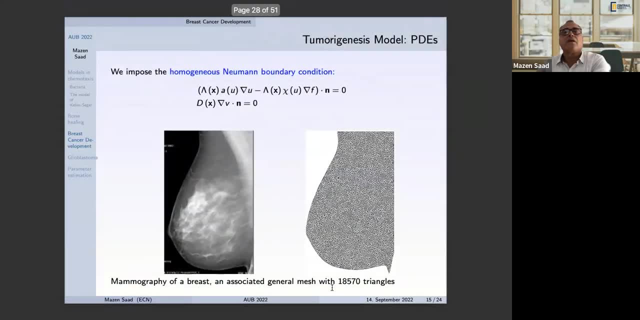 Okay, it is a complete model, Yeah, Okay. so now I want to show you only a numerical result. In our numerical scheme simulation we consider here that the breast is isolate, And so for that we consider there is no exchange between the breast. 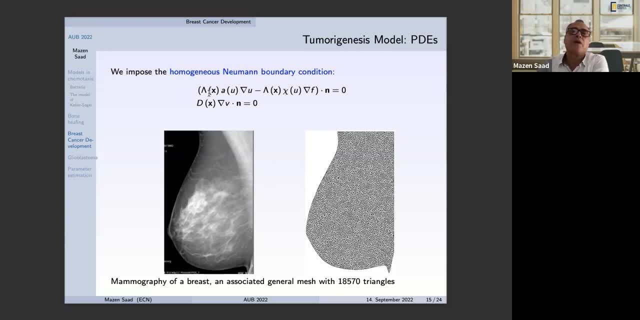 and the outside of the domain. Okay, And we write here not because we see a normal boundary condition. We use, as before here, the mammography of the breast to construct a mesh. according to this mammography And in our simulation here we have taken 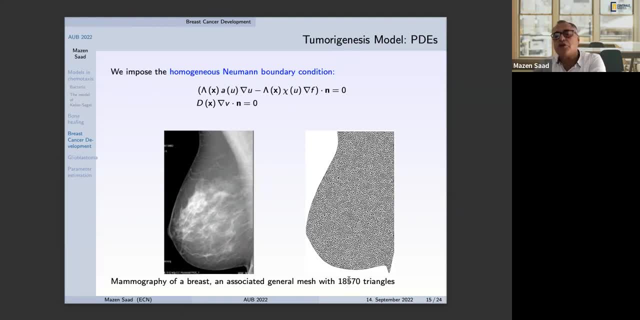 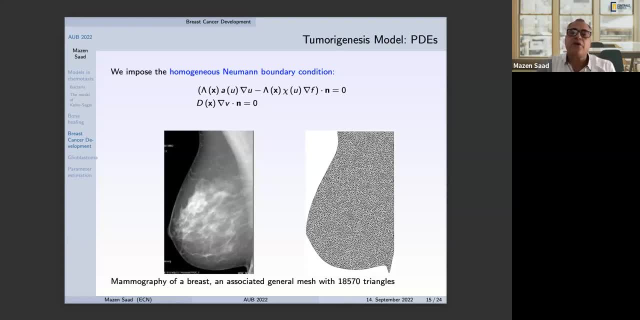 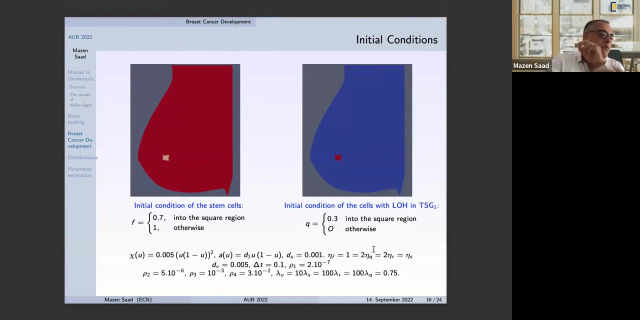 Which means the solution is very, very accurate For the initial condition. now we consider to an exceed to initiate evolution of the concept and we consider only: we consider only twoінandy-taidter, we consider only two溤or sних kiē is equal to one'allty'n 2021 candidate. 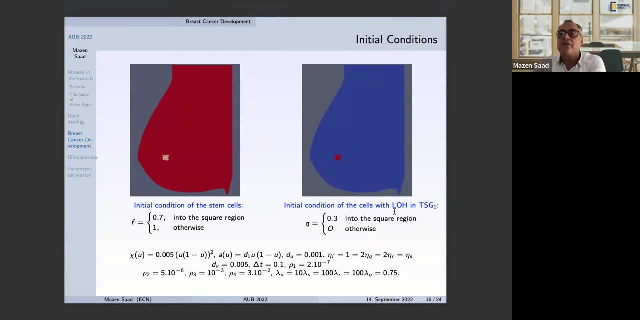 the initial condition with cells with the L-OH in only the first oncogen, T-SG1. And we consider that is equal 0.3 only in this red square region And we complete the initial condition for the stem cellular cells. 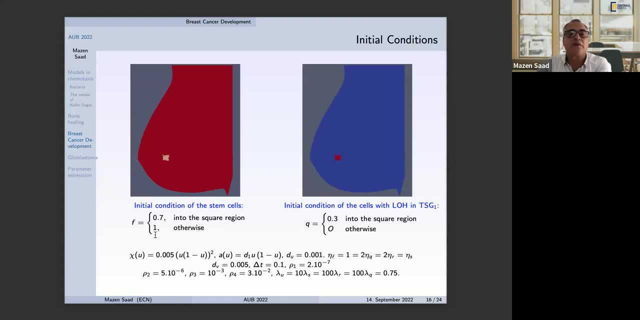 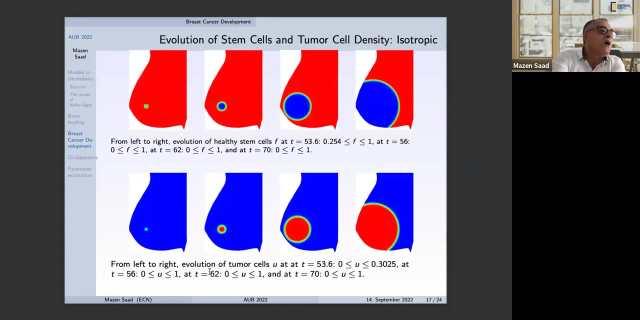 By taking the complement of this, one is 0.7 and 1.. Okay, And here there is a parameter. Okay, We have many parameters to do the simulation We draw here. the evolution of stem cells: Here is the time increasing. 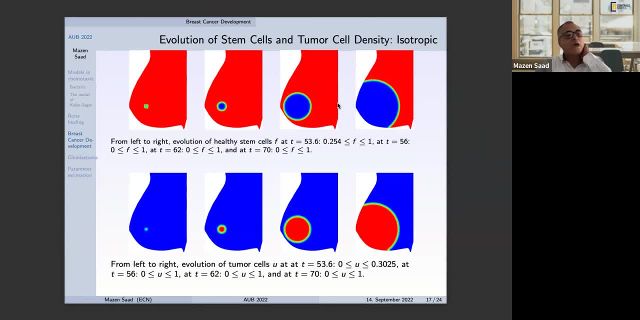 Okay, There is a time increase in this direction And we see here the destruction. In the first row, here we have the healthy stem cells And we see the destruction of the healthy tissue in favor of the evolution of the tumor cell. Okay, 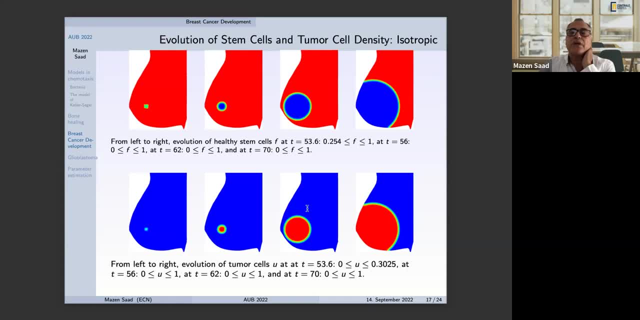 We have a concordance between the evolution of the healthy stem cells and the evolution of the tumor cell, Because tumor cells are attracted by the healthy cells, by the healthy cells. Okay, And here we have concerted, the breast is isotropic. 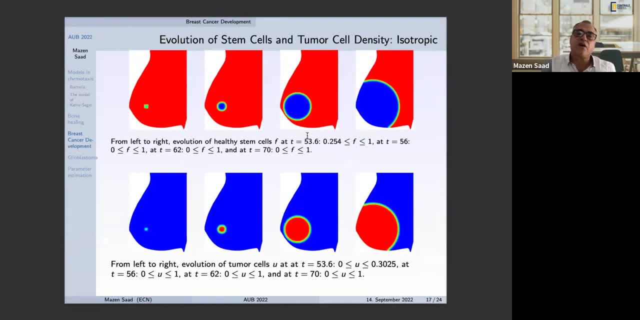 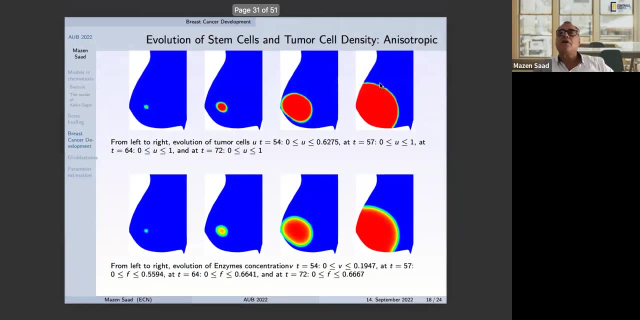 It is homogeneous. That means the direction, the diffusion direction, is the same in all direction And it's a constant. Okay, So to show, to illustrate the ability of our scheme to take into account the anisotropic of a medium, 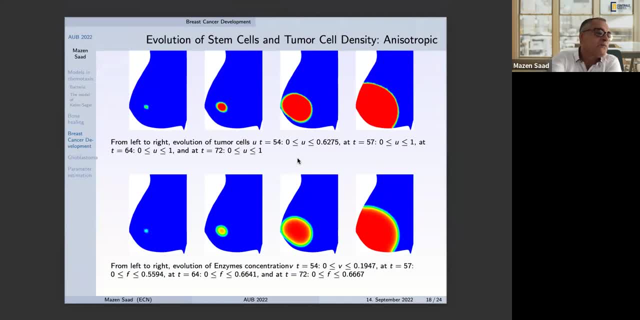 here we have considered anisotropic tensor in the diffusion, in the anisotropic of diffusion, the diffusion and the and the for the chemo-attractant part, And in this, this simulation, we see here the influence of the. 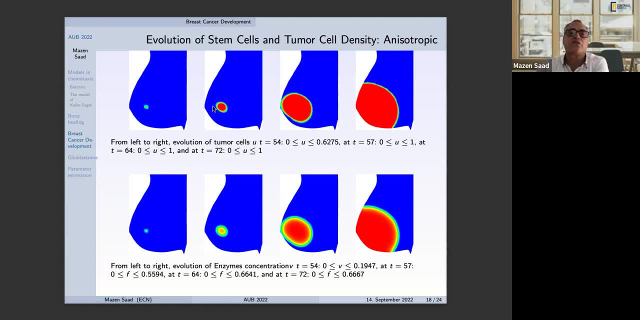 of the breast nipple, Okay, By taking anisotropic in this direction? Okay, And we see that here. I present here, in the second row here, the evolution of the enzymes concentration in time. Okay, So let's take a look at the effect of the two-phase. 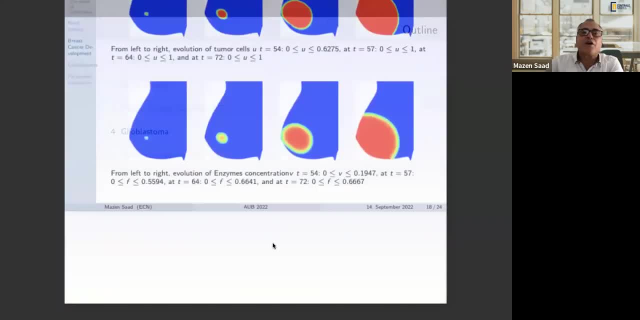 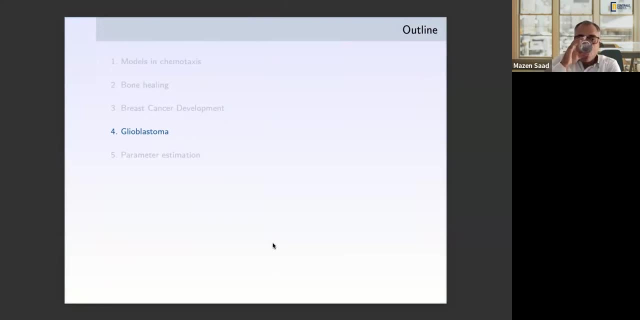 at the same time. Okay, Let's do this for the anisotropic portion In the same time. I have to take for the, the the two-phase for the anisotropic. we have been talking about the sequence and called this. 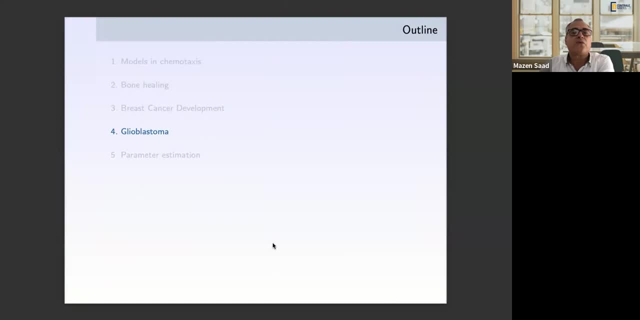 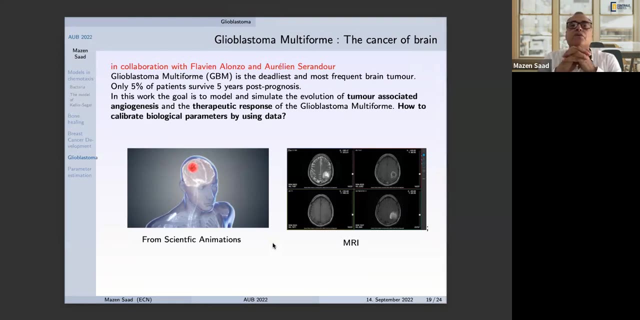 anisotropic by the your or the, by the, by the stress, but also this work in collaboration with Fabien Alonso and Aurien Serandour. glioma multiforme JBM is the most frequent brain cancer and only five percent of patients survive five years. 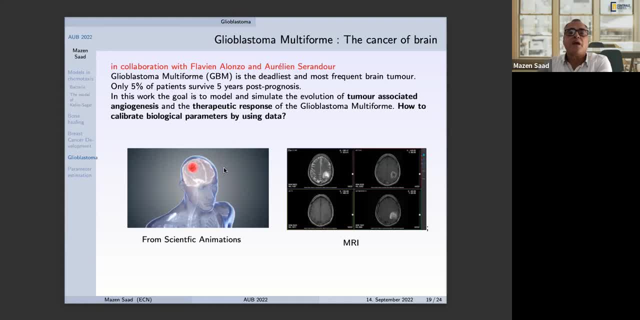 post-progenesis In this work. here we are interested in the modeling and the simulation of the evolution of the tumor brain. and we add here: we are interested also in the therapeutic response to the treatment. We add here the treatment by surgery, chemotherapy and radiotherapy. And finally we are interested how to calibrate. 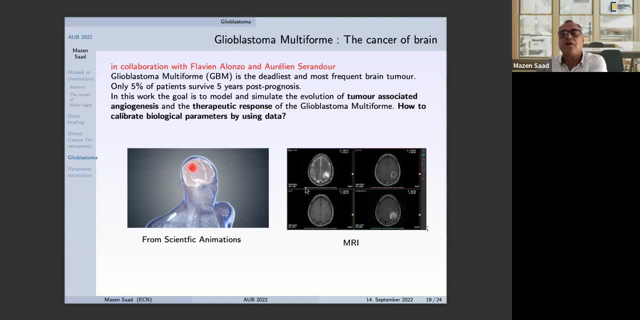 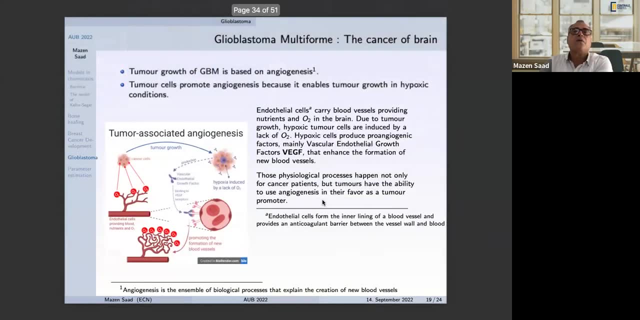 the biological parameters by using data, For example the MRI here, Okay- as other examples. I begin here by by explaining in my word the biological process for this tumor. The tumor growth of JBM, of the glioblastoma, is based mainly in angiogenesis and here the tumor cells 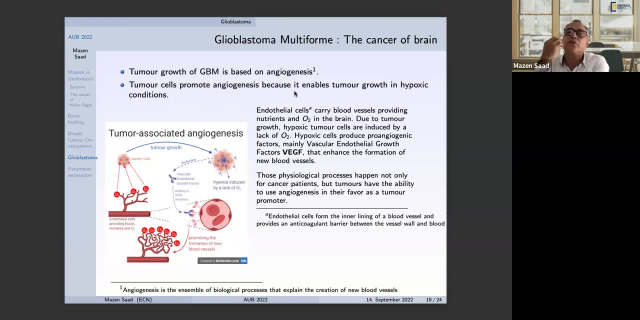 promote an angiogenesis because it enables tumor growth in hypoxic condition. I explain here in this scheme, the mechanism of the tumor angiogenesis. firstly, the endothelial cells. the endothelial cells carry out blood vessels, providing nutrients and oxygen in 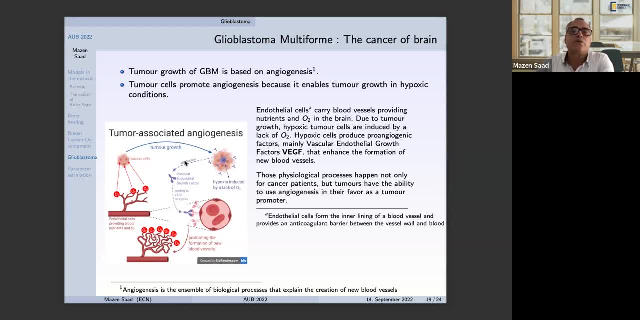 the brain due to the tumor growth. hypoxic tumor cells are induced by the lack of oxygen. Hypoxic cells produce the production of proangiogenic factors and these factors are the vascular endothelial growth factors. they do not VEGF and this enhances the formation of new blood. 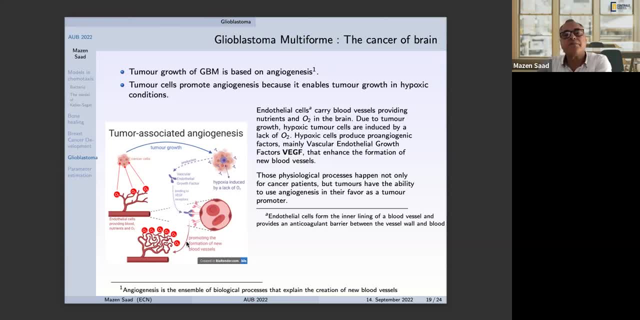 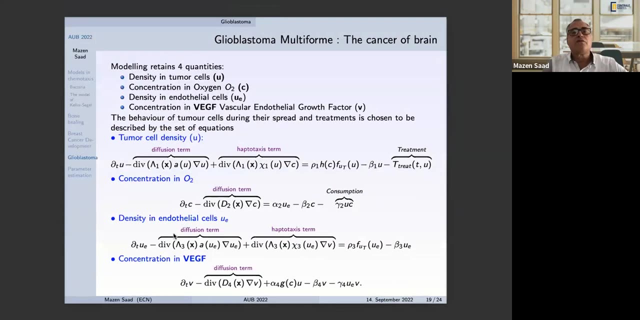 vessels. Okay, It is a mechanism here to To explain the development of the glioblastoma, For the modeling for this problem. the modeling we retain here: four quantities: the density in tumor cells and the concentration in oxygen. Okay, 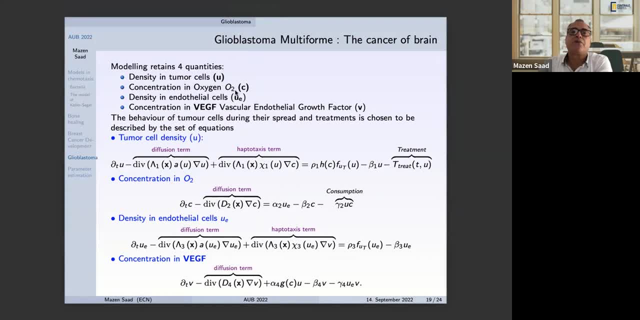 It is In general. In many people they use this simplified model, but here, in order to exhibit angiogenesis, two quantities are added into our model: the density of the endothelial cells and the concentration in the vascular endothelial growth factor. 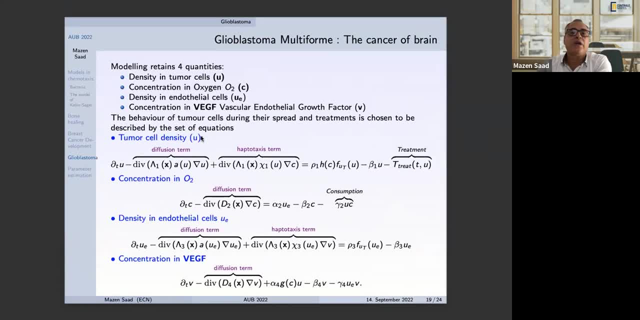 Okay, Okay, So we Here we are in the. We are in the presence of two systems of keratogenes and the two systems are copied. okay, It is classical. here for the tumor cell density, we have the diffusion and the apotaxis cell. 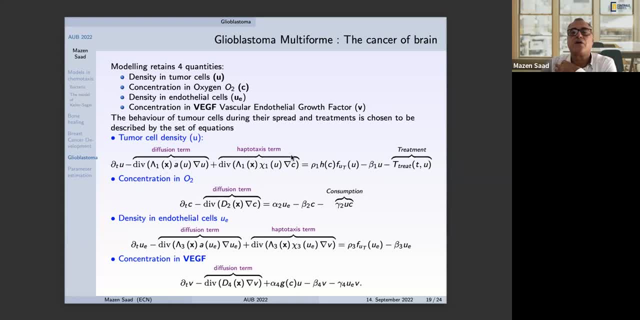 due to the high gradient of the concentration. Okay, Okay, Okay, So we have the diffusion and the apotaxis cell. due to the high gradient of the concentration of the oxygen, And in this model- okay, this is a classical reaction. then we add here the treatment of: 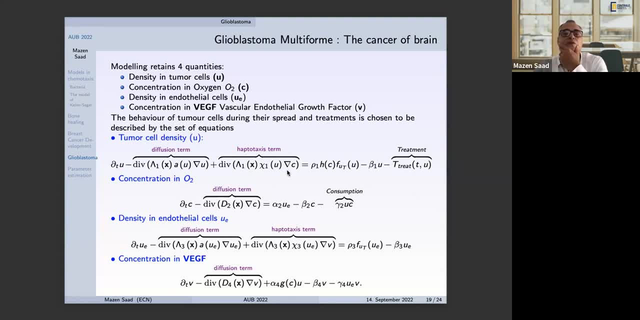 this Of the tumor. Okay, We have the concentration. We add here the consumption of oxygen by the tumor and also for the density of the endothelial cells and VGA. We have also the, We have the diffusion term, and the endothelial cells here are attracted to the high concentration. 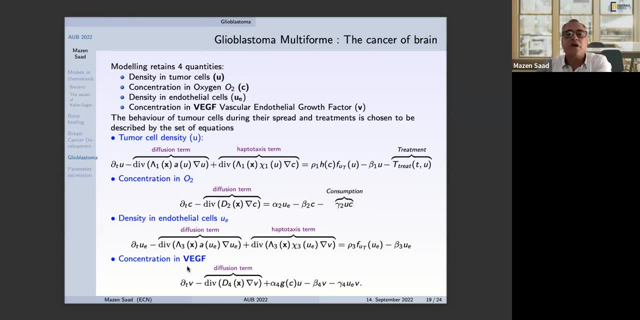 in the growth factor of the vascular endothelium. Okay, And here this is equal. Okay, And we see here the Okay, Okay, Okay, Okay, Okay, Okay. So we see here the linking between this model and the evolution of the tumor cell. 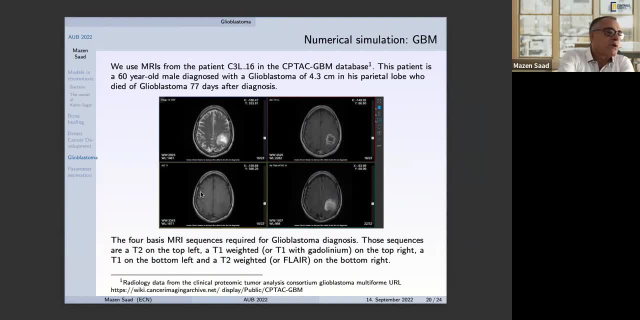 Okay For our numerical result. we use here MRI for a patient And we use here a free database. databases we have here. if you are interested by this database and this database, we have the mri sequence for many, many, many patients and here we consider a. 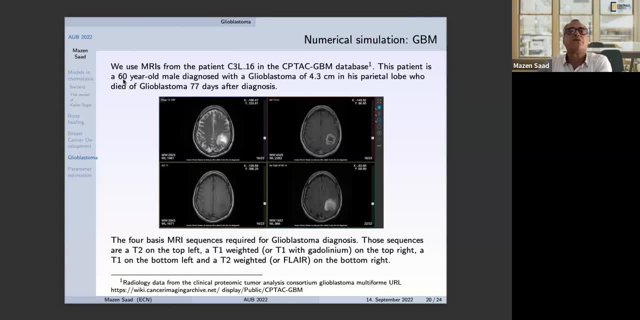 a patient with he's 60 years old and with a glioplastoma of 4.3 centimeter here. okay, and it is the same. it's the same, mri, but in in different, in different sequence. because we can add, we can inject here gadolinium to show the tumor in different, different way. okay to for our numerical. 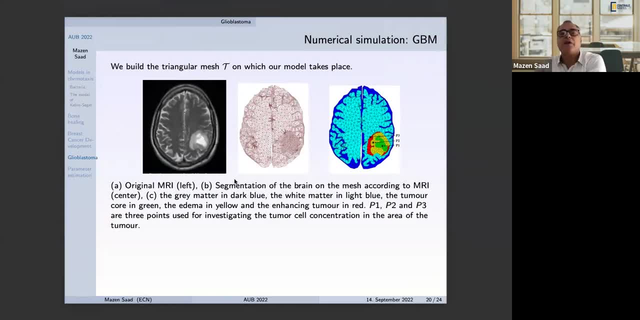 solution we consider: here is our general mri and next we construct a segmentation of the brain on the mesh according to this mri and in the domain here the the brain is is the tropic. the gray matter here is in in dark blue and the white matter here in light in light blue. and next to impose the initial condition and take 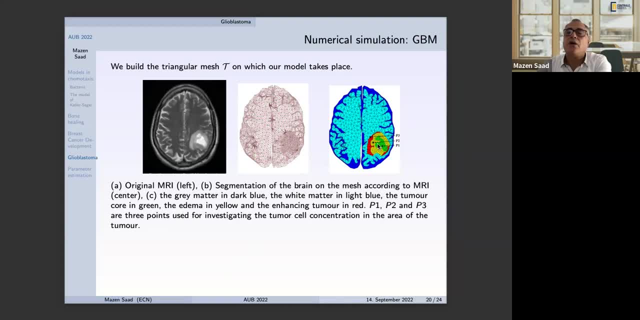 into account of this, the steamer. here we have three, three region, the. the core here in, in green it is a, it is the tumor, the edema here in yellow and finally in red, it can be considered, as you see that the flare as a flare of of the tumor. 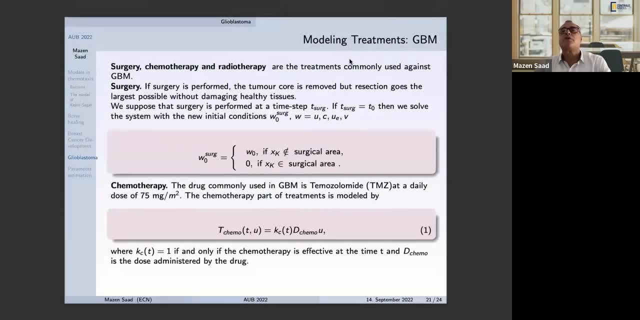 okay, i focus now to the modeling of the treatment we take into account here. surgery, chemotherapy and radiotherapy are the the treatment commonly used for gbm surgery. eh is very is very simple. madfonit core point of view code here is removed and we consider that all quantity. 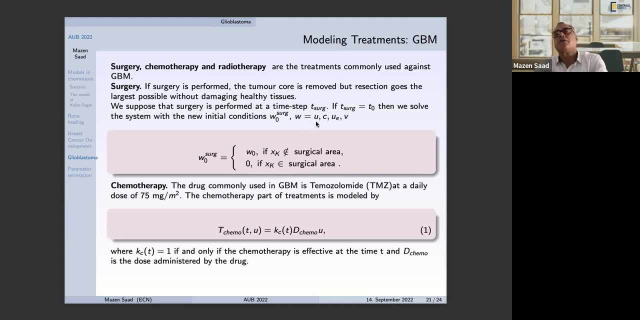 a quantity of density of the tumor that we라고 is life and weight of the tumor here, and we consider all quantity, the density of the tumor. here we take into account and uh, then and then if we dancing patient diseases w and we consider that all the opportunities outside of now. if there is an expression means that if the tumor free production it is not él定 in detail in the and we consider that all the opportunities outside of now if there is an expectation. the Doncaer came into theх. 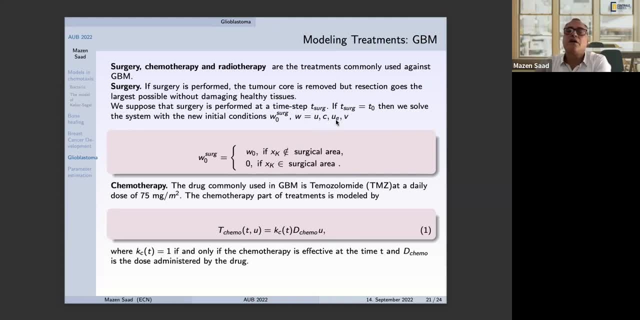 tumor cells, the concentration of oxygen for on the territorial cells, etc. all these quantities are removed and we consider zero in the surgical area. in the other, in the other area, for the rest of the brain, we consider the same, the same solution. or in cell condition for chemotherapy we use the protocol used in france. and here's a drug. 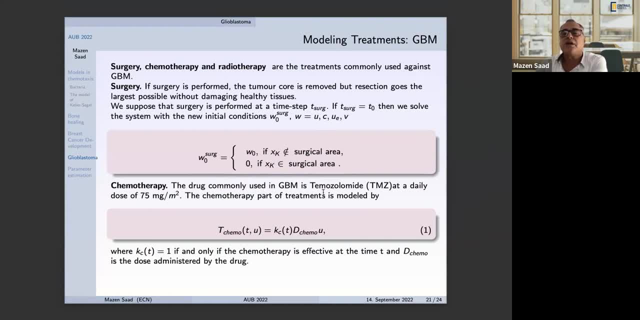 commonly injected here is a timo, is the tomolomozid, it is tmz, and then, mathematical point of view, we add the, only the dose, the dose of the drug administered by the drug, and if the chemo therapy is effective at time t, maybe with this term. 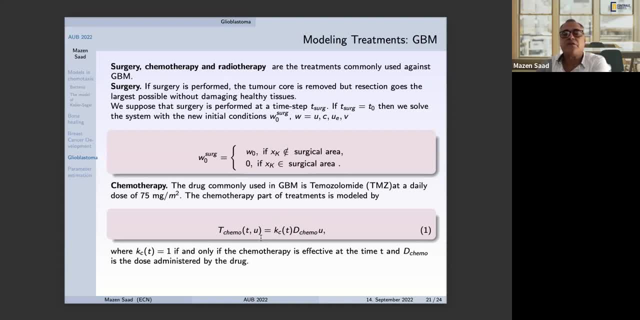 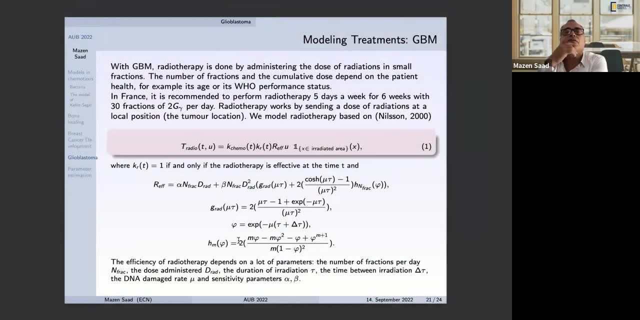 multiplied by the dose of administration, and this term is a source in the equation. and finally, for the radiotherapy in france, it is recommended recommended to perform radiotherapy therapy five days a week for six weeks, with some fraction, with here we consider 30 fraction of two of two grains per day. 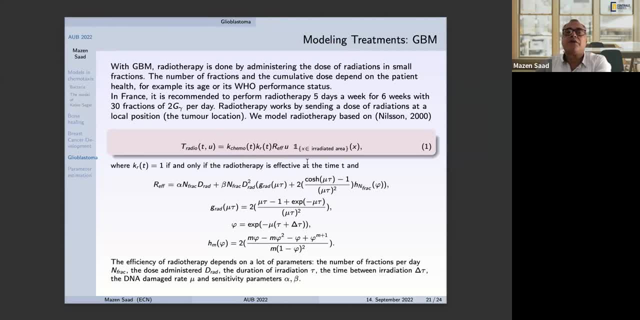 and to model this radiotherapy work is by by sending a dose of radio radiation only at local position. so in this, in this equation, we we impose the radiotherapy only in the irradiated term. okay, and for the model of radiotherapy, the model is very, very complicated. 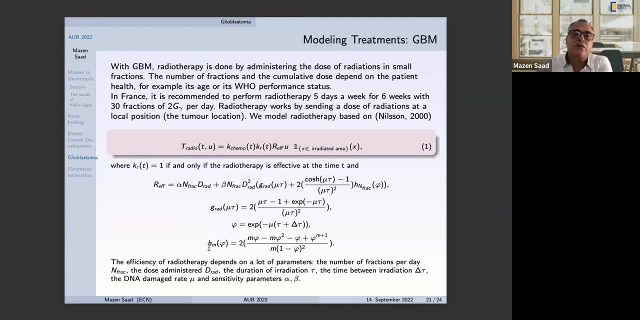 because the efficiency of radio therapy depends on the radiation and the radiation is very, very. The efficiency of radiotherapy depends on a lot of parameters, depends on the dose administrated, the duration of irradiation and this function over here we have many, many parameters: alpha, beta, mu, et cetera. 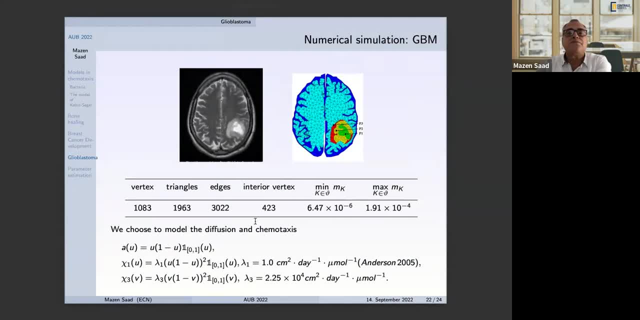 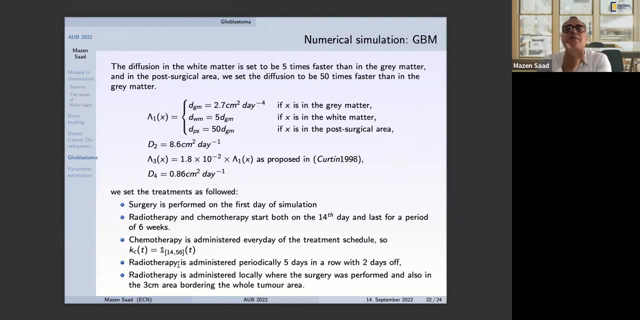 Okay, here I give you only the number of set triangles for this simulation, which is about 2,000 triangles. Here is some data. The brain is not symmetric. The diffusion coefficients are not the same. We consider in the white matter here is that the coefficient of this diffusion is said to be five times faster than the gray matter. 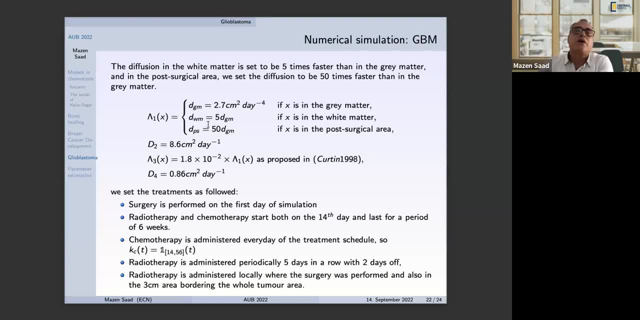 And in the region where the post-surgical area, here there is now nothing and we said here the diffusion in DPS here to be 50 times faster. Then the gray matter diffusion coefficient. We apply here the protocol as we used here in France. 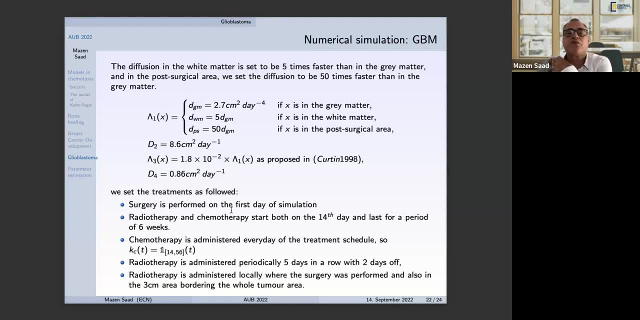 We consider surgery is performed for our simulation at the first day of simulation. Okay, we start with that. Then radiotherapy and chemo therapy start both in two weeks, 14 days after the surgery, and last for a period of six weeks. 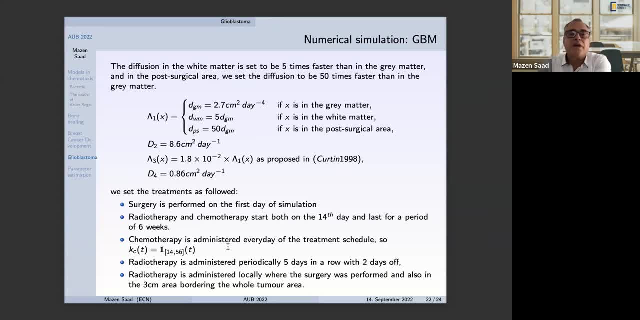 And chemo therapy is administrated every day And okay, radiotherapy is okay. Okay, And chemo therapy is okay In general also, the radiotherapy is administrated locally and also around the area region: three centimeter area boarding the whole tumor area. 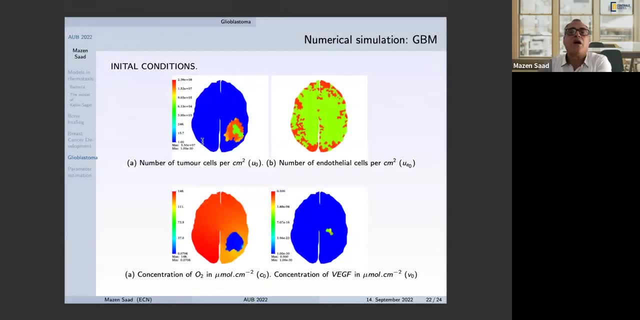 Okay, I show you here the number of the initial condition, the number of tumor cells, the number of endothelial cells. Okay, it's not the same In gray and white matter. Okay, for the concentration for oxygen and DHA. 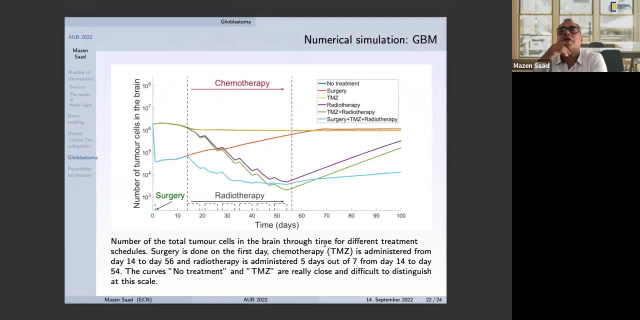 Here I present you only this graph for this numerical simulation In the y-axis. here we have the number of tumor cells in the brain. This is a global number, the global number of the total number of cells versus time. And here we have do many simulation. 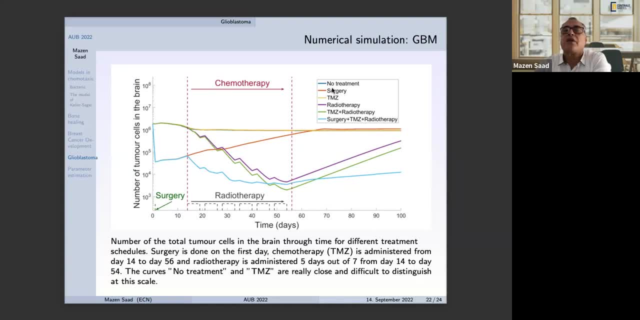 With the first one we do nothing, no treatment, And here we do surgery. TMZ is chemo therapy, radiotherapy is a combination with chemo therapy, radiotherapy, and also we have surgery. The first command is: the curve is here. 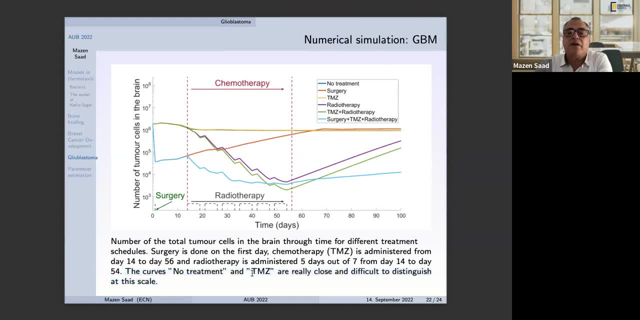 No treatment And chemo therapy are exactly or very, very close, and so it's difficult to distinguish at this scale. It is this curve in orange: Okay, no treatment and TMZ are the same, And this conclusion says that for all the patient. 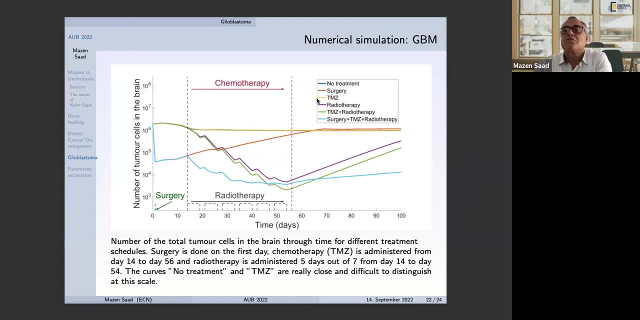 it's not necessary to give chemo therapy only because you have the same result as do nothing. nothing Okay. Next, you take surgery. Surgery is good. okay, because the number of tumor cells decreased And after that continue to increase, continue to increase, okay. 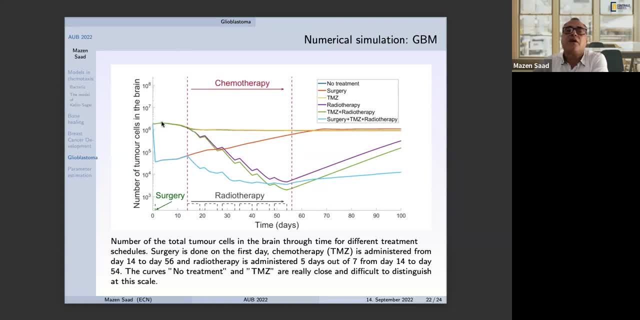 If you take radiotherapy, radiotherapy is very, is very efficient. Okay, in this period here we have radiotherapy. Okay and very. but when we stop radiotherapy, the number of tumor cells increased, Increase, increase. And if you combine chemo therapy and radiotherapy here, the result is better. 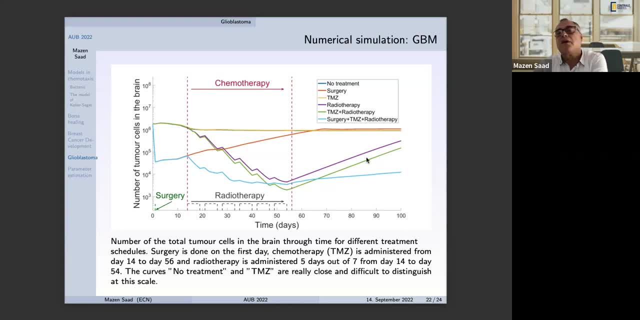 But when we stop the treatment we have also the number of tumor cells increase. The best here treatment is to combine surgery, Chemotherapy and radiotherapy. We see here in this point that when we combine this curve is better than the other. 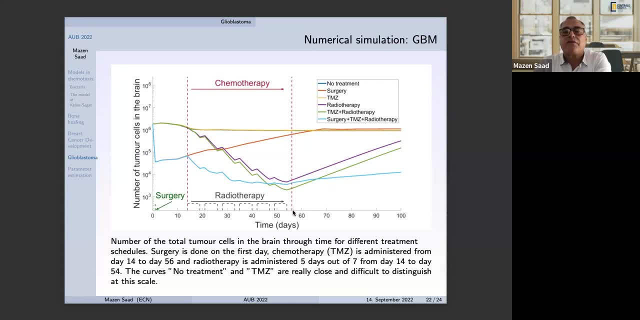 The number of tumor decrease. And when we stop here after, I think, 56 days, the number of tumor cell remains constant. okay, There is no decrease, no increasing as before. And for this tumor the combination of the three treatment is good. 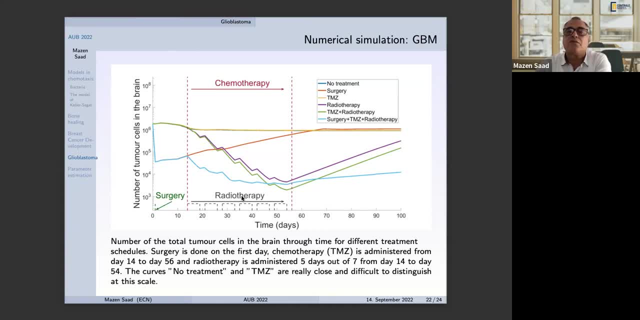 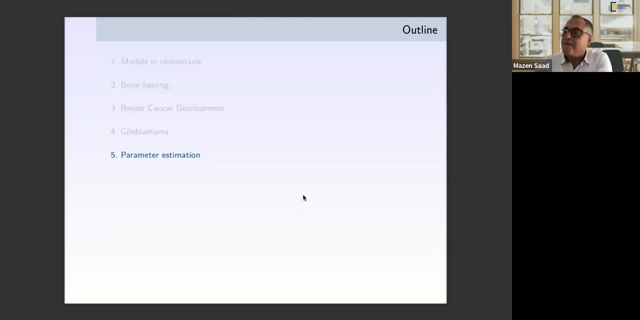 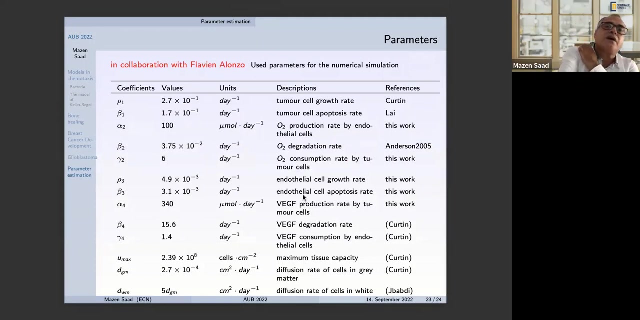 And this protocol. it seems good. Okay, I have, I take two minutes, three minutes to explain, Okay, yes, Yeah, okay, thank you. In to do the our numerical simulation, we have used parameters. okay, 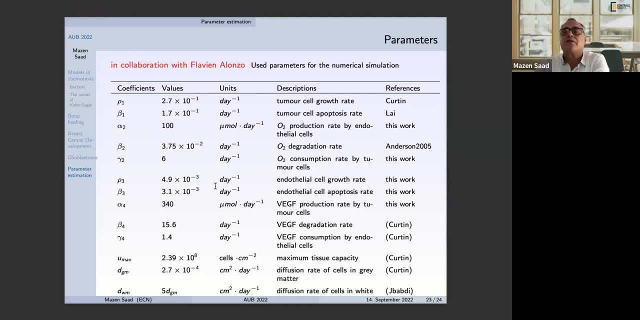 And we have very, very many parameters In the literature. We take, for example, this value by considering here this article. Okay, it's very, and you can see that this parameter depends on the, on the referee And the. the question which we ask is: 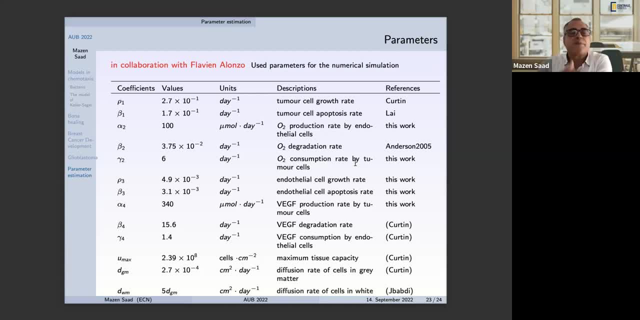 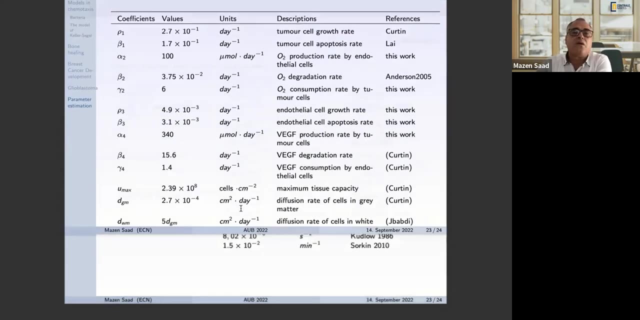 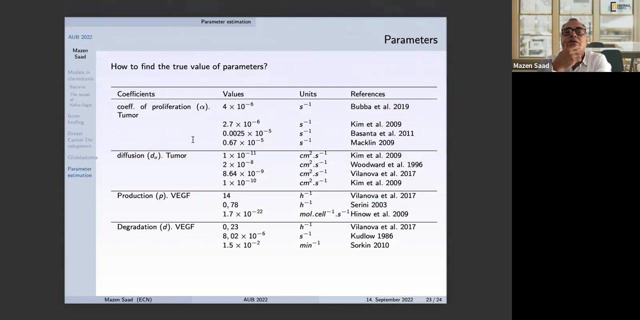 the question which we ask here are: these parameters are are true, And what are the the right parameters? If you take, you have a patient, what is, what are the parameters? Okay, Okay, We don't know how to find the true parameters for a patient. 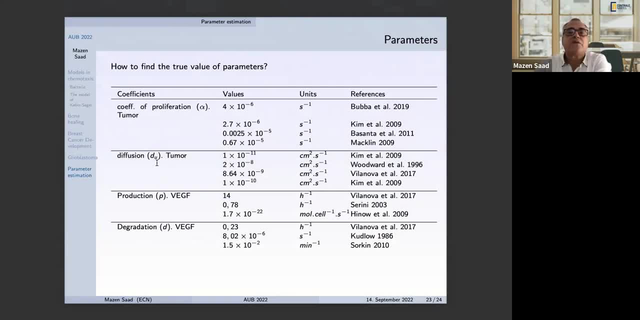 For example, if you take here the diffusion coefficient for the tumor, the, the value is very, very different. It depends on the order. It is the same units, but it is if you take the 10 power minus 11 and 10 minus minus 8,. 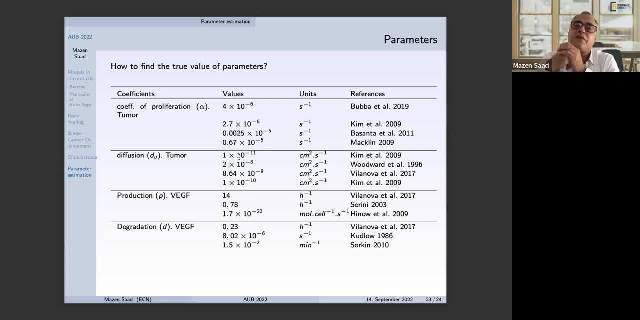 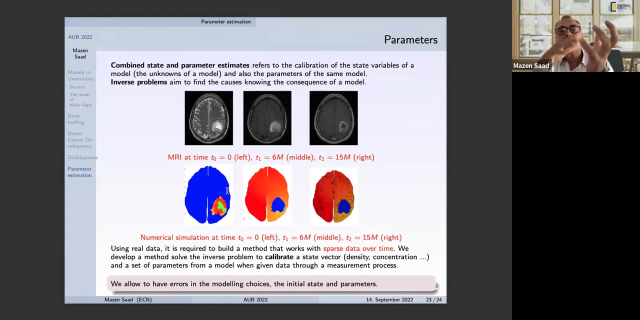 the spread of tumor is not the same. It's not the same. Okay, And and so we are. we are interested by the question: what are the right parameters Here? in this project, we we try to calibrate the state variable. 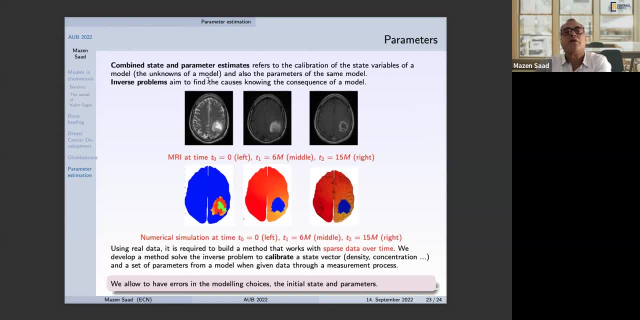 meaning the unknown of the unknown of a model and also the parameter of the same model. Okay, The same parameter is not, we don't know exactly what it is. Okay, We have a construct here, a model, And the model in for the numerical simulation produce the same phenomena. 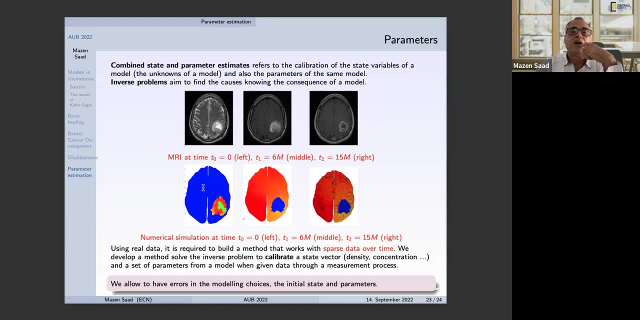 Okay, We say that the the figures here are are the same or or very close. Okay, We have a doc here on on our model. Our initial condition are not good also, And we don't know the parameters. And here we want to use real data to ameliorate or to calibrate our model, the parameters and the initial condition. 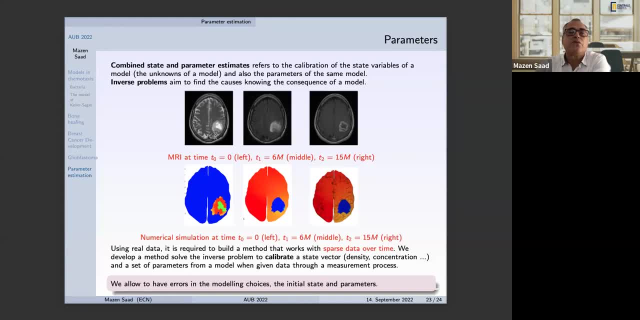 And this, this problem is complicated. Thus, if you want to use real data, for example MRI, you have some MRI at 0, T after 6 months, 15 months, et cetera, And we need here to, to, to to work, a method that works with sparse data over time. 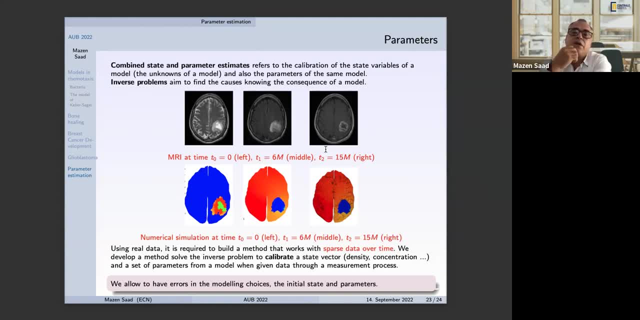 Okay, Because you have. you don't have the information at any time and also at any space, Because if you have MRI or analysis, it's not possible to have the value of the locally, the value of of the cell, of the cell density, of the concentration on oxygen, et cetera, and the parameters. 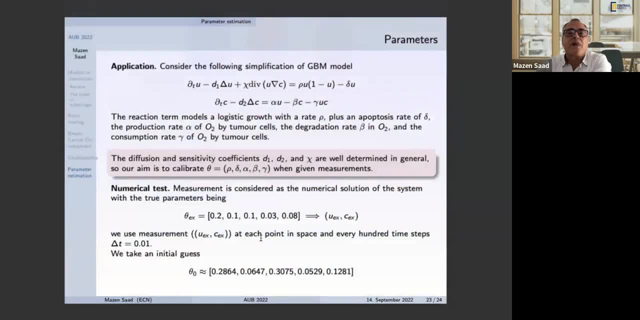 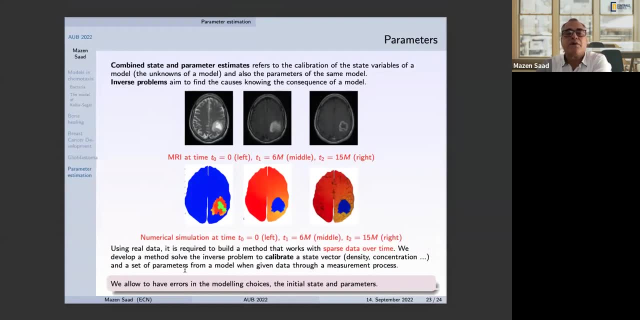 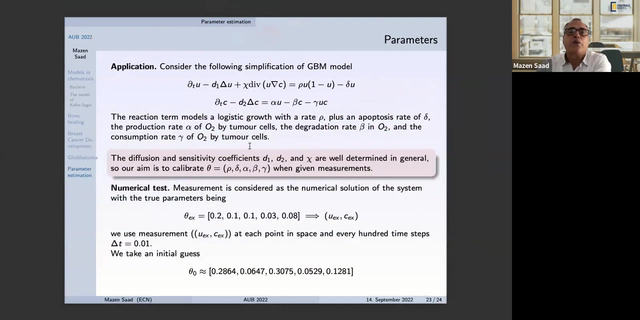 Okay, We have many errors here. It is this problem we, we, we have to solve an inverse problem: to calibrate the parameter and the model. Here we, we try our method by: by using the, a simplified model of GDM. 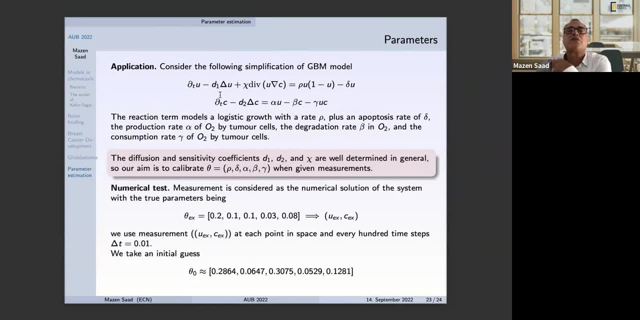 We consider only the concentration of the oxygen. Okay, Okay, We know the concentration of the oxygen in a tumor cell And, in mathematical point of view, we aim to to find the parameter, the parameter only for the reaction term: rho, delta, alpha, beta, gamma. 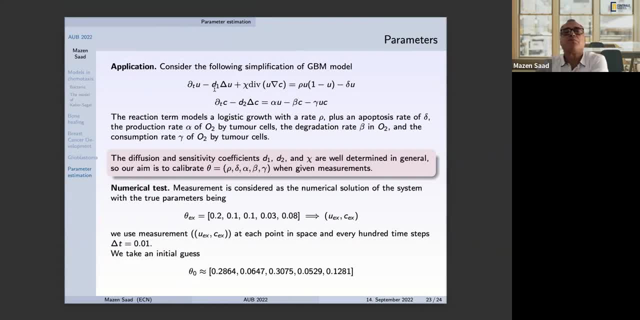 And here in, in this method, we, we suppose that the diffusion coefficient and the chemotactic coefficient is, is, is given, Okay. Okay, we start by to validate our method. we consider, we look for this parameter, theta, exact. here, for example, you give this number 0,, 2,, 4,, rho, etc. 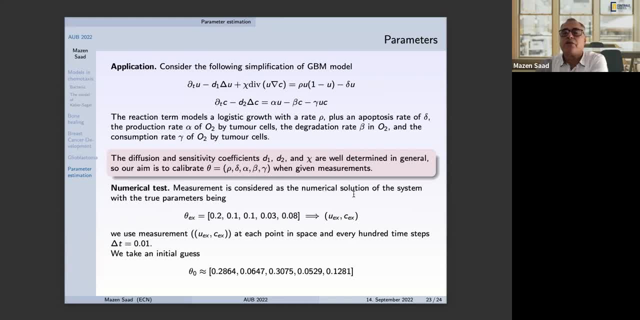 And we compute the numerical solution associated to this parameter. Okay, and here's the exercise. Now we forget the theta exact, the parameter, because in general we don't know what is the parameter. What we know here is observation. For example, it's equivalent to MRI. We have the solution u and c at any time in each point in the space. 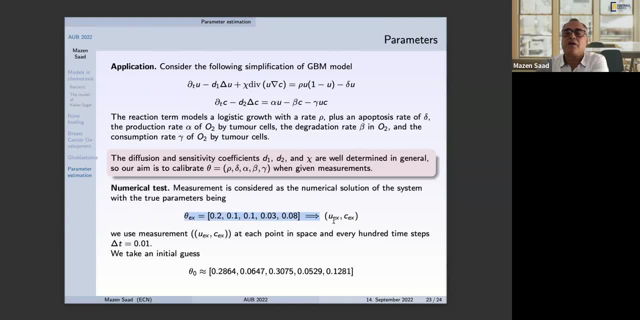 And in this part we don't know what is the parameter. We have only the consequence of this simulation. It's exactly the definition of the inverse problem. You have here the solution, but we don't know what are the parameters. Okay, and we consider here the observation: or the law: are the solution computed by this exact solution? 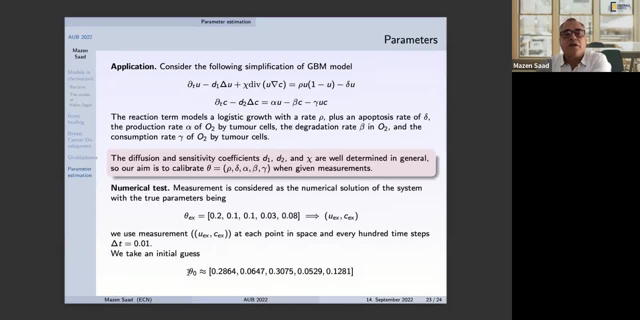 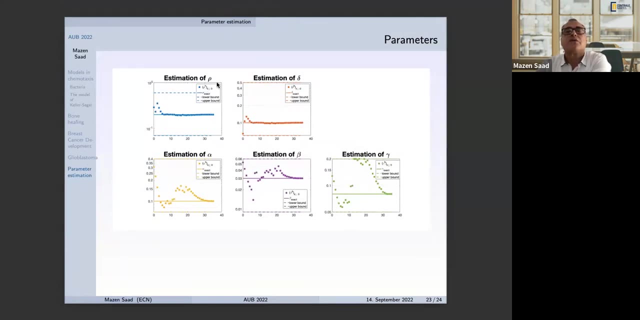 Okay, And we start. We start here with initial guess, theta zero. It's not the theta exact, It's different from this one. And we solve our inverse problem to construct a numerical sequence for all parameters And the parameter. here we see that by solving this problem we find the parameter, the expected parameter. 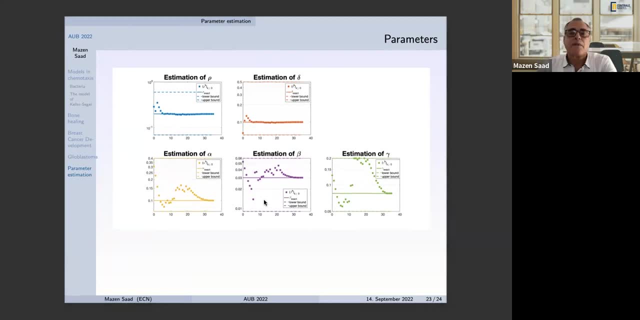 And we do the same thing here in the continuous line. Okay, but this problem is an open problem for us And to apply this inverse problem of the calibration for the glioblastoma, it's not easy to do that because we have many, many missing data. 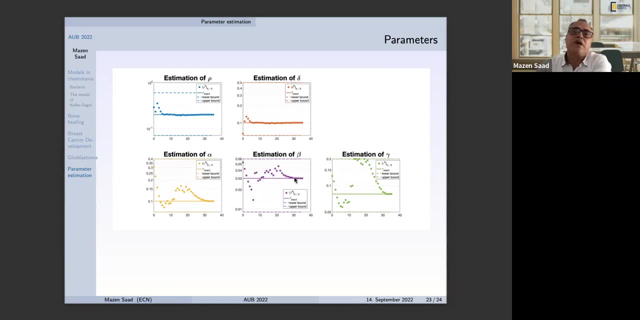 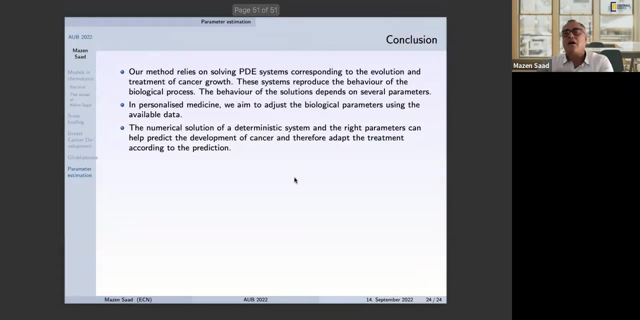 okay, here we. it's possible to do that because we have the exact solution. okay, in conclusion of this, this talk, our, our method, or our numerical method, and modeling here relies on solving partial differential equations system which corresponding to the evolution and the treatment of the certain concept. 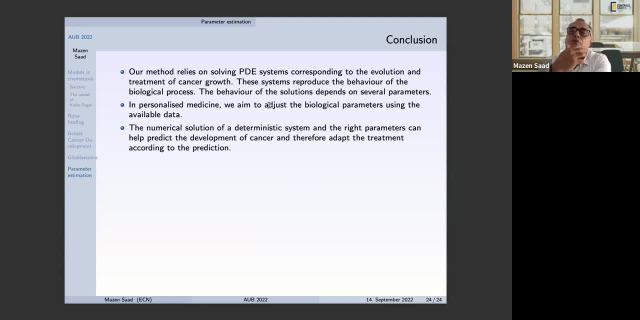 this system reproduce the behavior of the biological process and but the behavior of this solution depends on several parameters. in personalized medicine we we aim to adjust the biological parameter using the available data and in in our approach we use only here's a numerical solution of a deterministic system. okay, and the right parameter can can help. 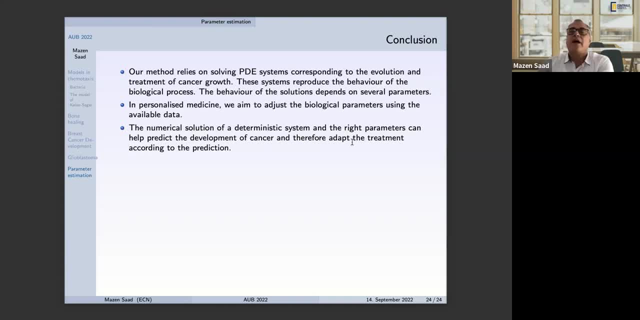 predict the development of the cancer and therefore adapt the treatment according to, to you, this prediction. okay, it's our aim, but okay, we we try to to give a short answer of this problem and thank you very much. thank you, thank you very much for this interesting talk. uh, well, it's time for. 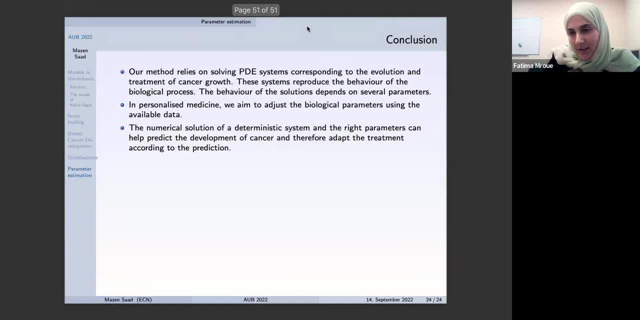 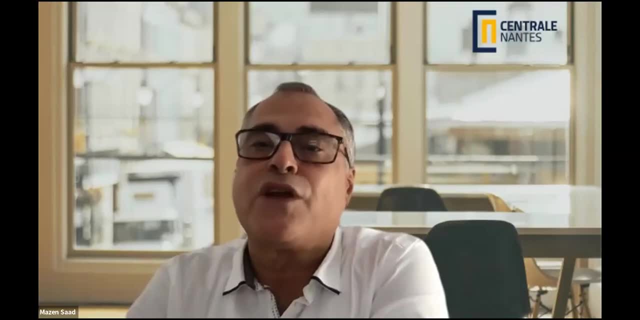 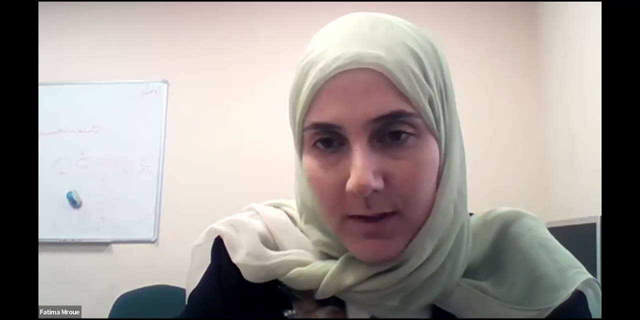 questions. i think we can receive a few questions, so any questions from the audience. okay, they can write my church the. they can write my church the question either does the question either by chat or raise hand to ask the question directly, or unmute themselves and ask the question directly. okay, 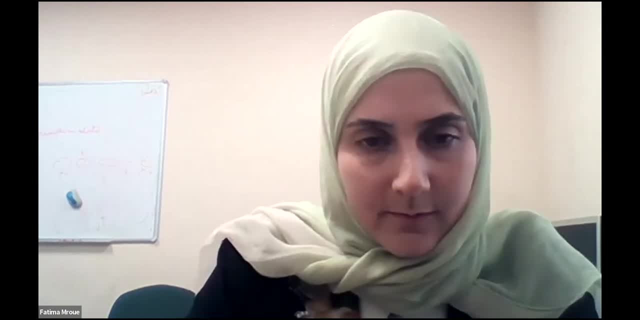 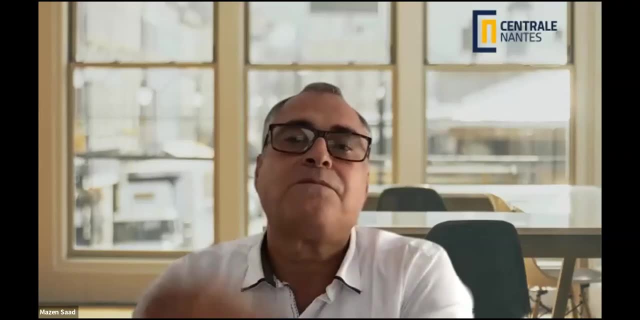 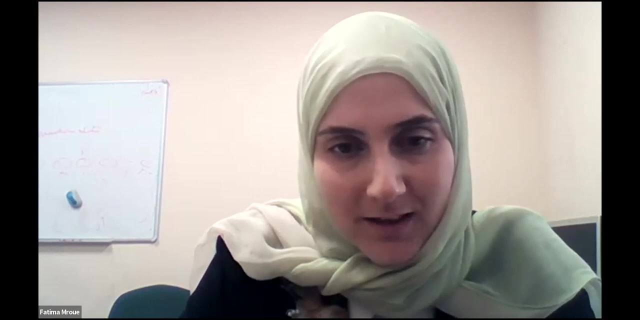 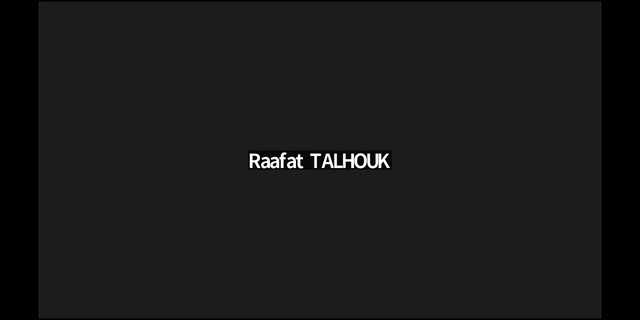 well, i don't see any raised hands. okay, well, okay, so okay, i, i have one raised hand. uh, professor, can you please uh unmute yourself? uh, hello everybody. thank you for this interesting project, for all what you want to present in this series of uh similar concerning biological mathematical village. thank you, uh, professor mason, for this. 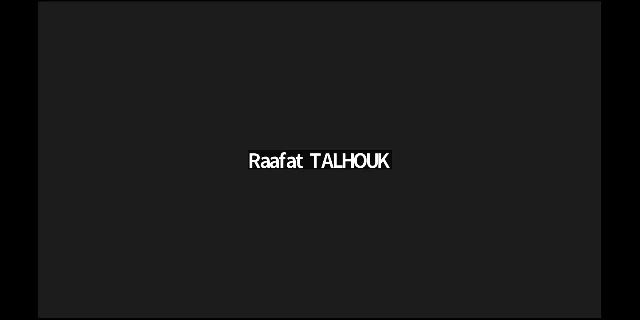 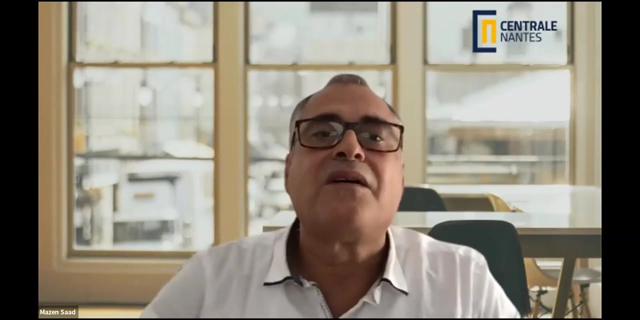 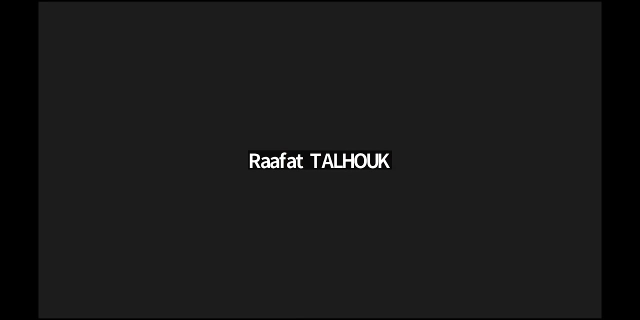 nice thoughts and very rich. i have one question, just one question, concerning the mathematical systems. um modeling the best concepts. yeah, i see that it is a very complicated and is performed by copying uh many differential equation, ordinary differential equation with pdes. yeah, with the color cycle model, i guess. and you have talked about numerical results. 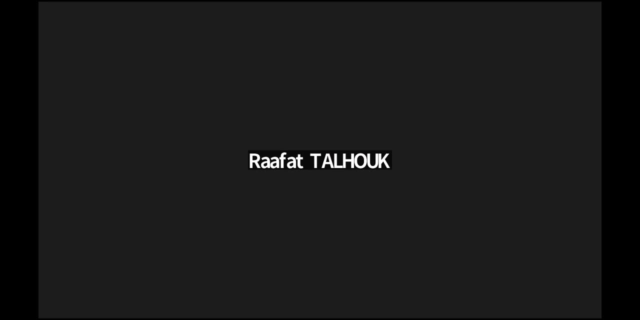 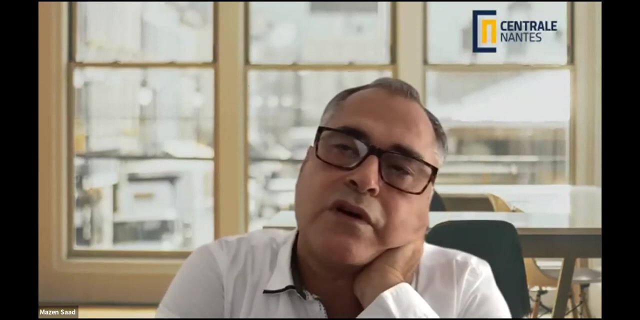 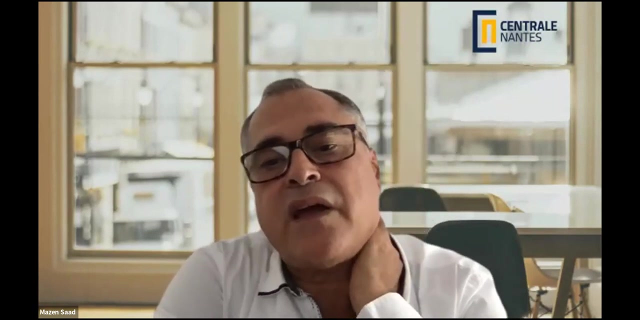 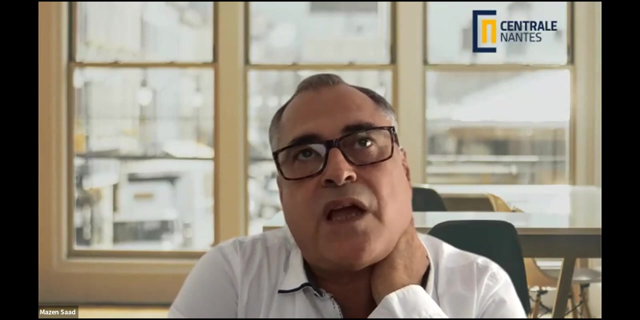 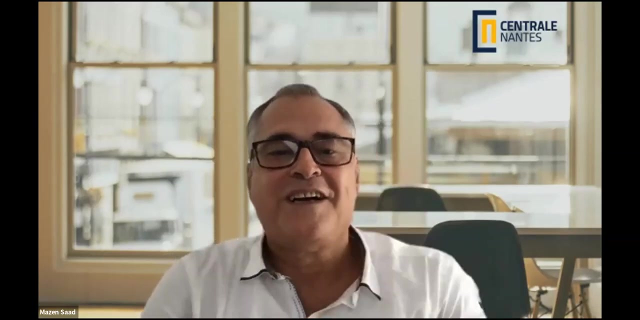 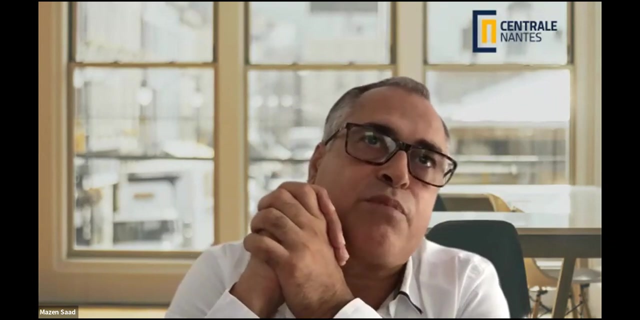 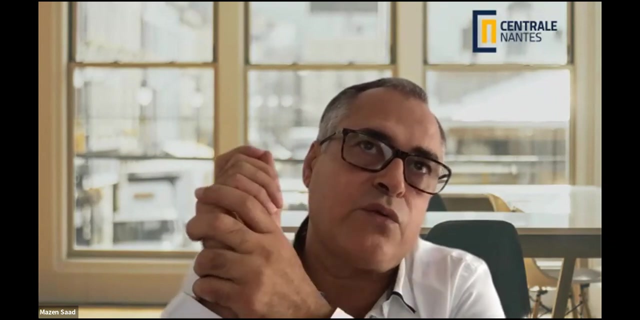 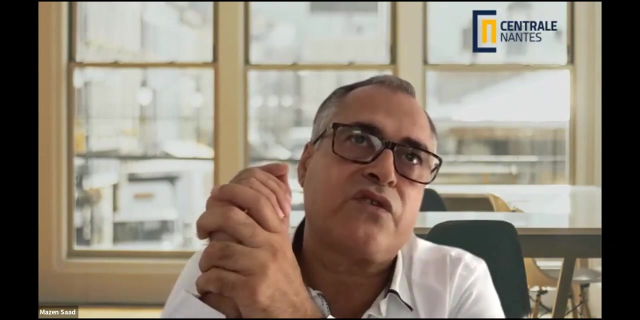 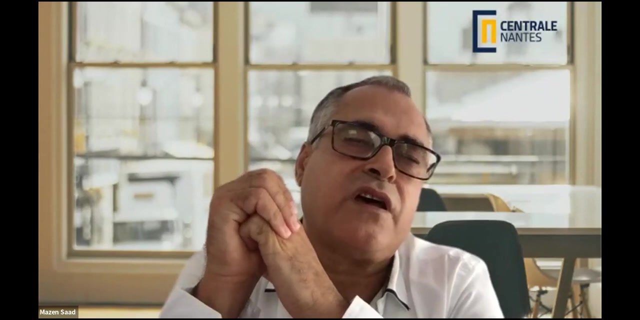 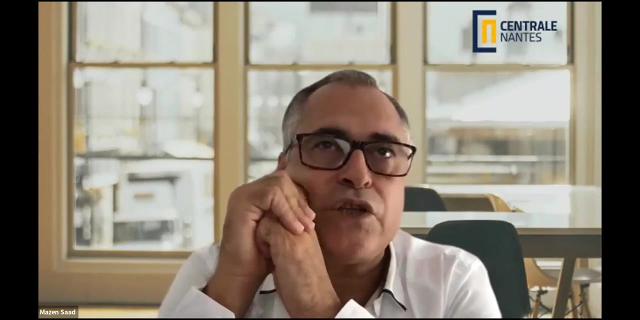 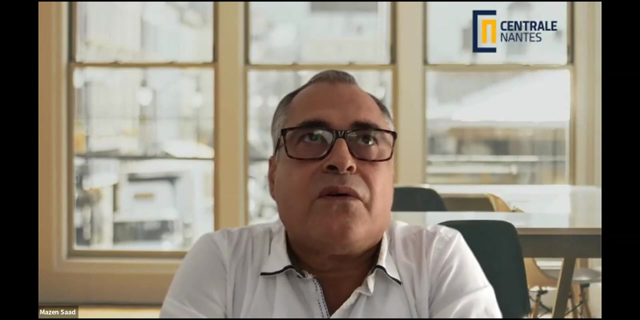 my question is concerning, uh, what about mathematical results, and particularly maybe the uh, uh, uh, uh, uh, uh, uh, existence of the global solution, of this assistance, uh, of this system, okay, and and what about the regularity and the of the concentration of enzymes is positive and the solution is in l2, h1, l2, h1 and it's all okay. 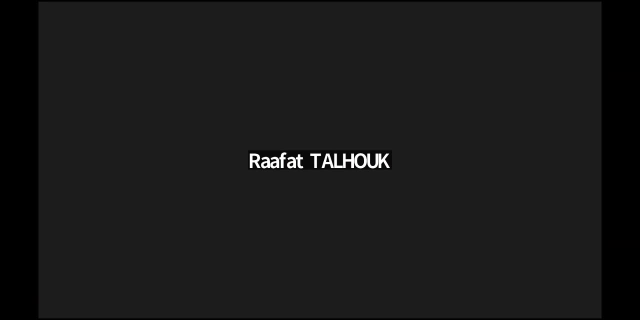 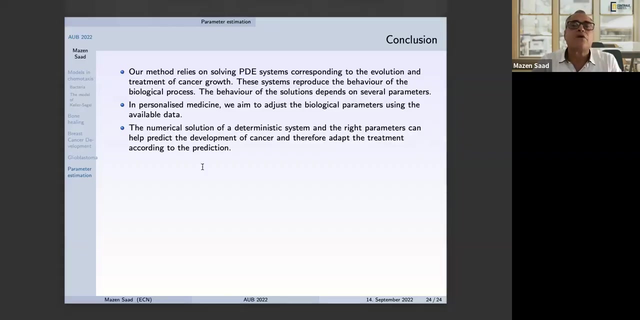 and this means that you have the maximum. it's a maximum principle. i have the maximum principle for all quantities and i can write it. and what uh, what, numerically also, you can uh verify the, the maximum we, we can uh uh preserve the maximal. yeah, yeah, i present we, we choose. 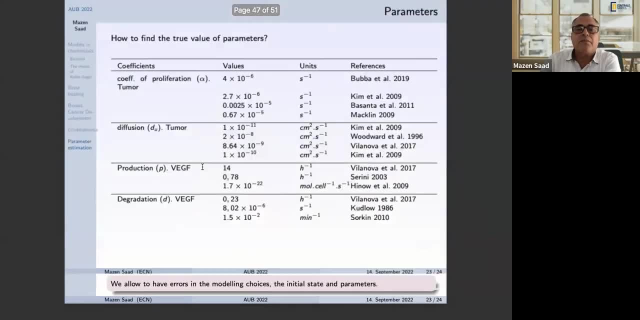 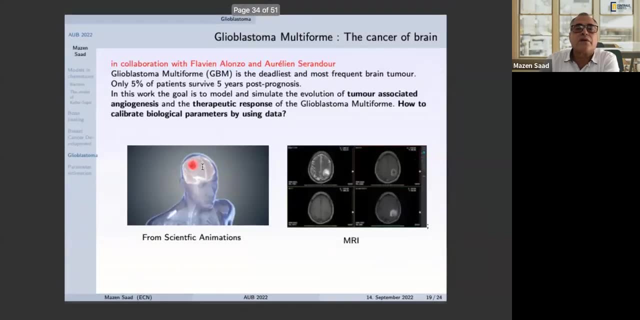 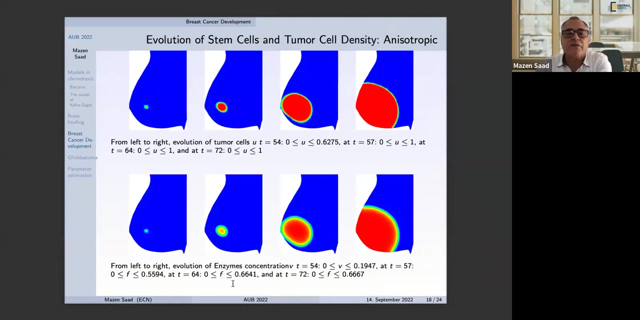 we choose our scheme, preserve the maximum principle and we show, we show here, and i think i put here and here we have: for example, v is between zero and one, f, we, we preserve the maximum principle for all quantities and u here is between zero and one. good, okay, in the same mood: uh, what about the system in appearing in geo plus toma? 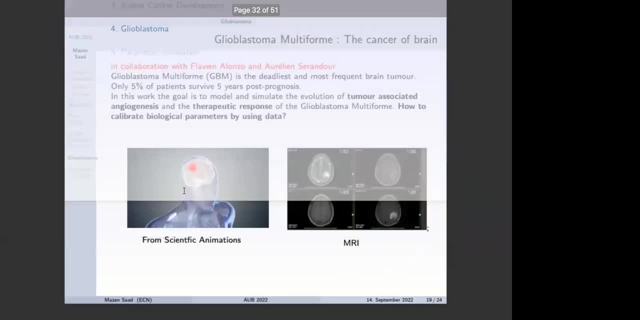 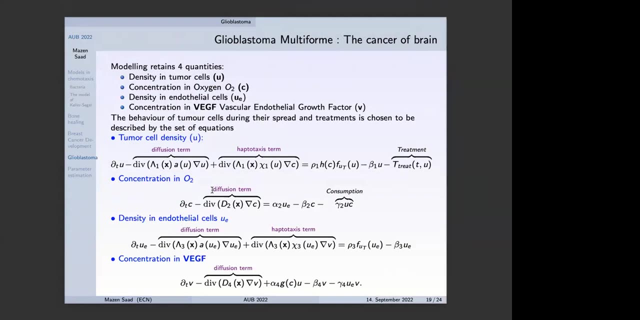 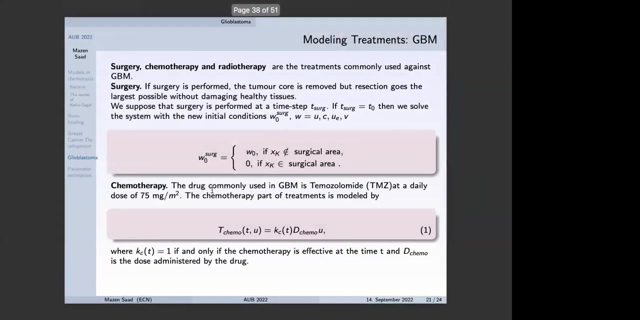 because here i i i see that you have endocatrics function in the system and maybe you have some singularities. do you preserve also mathematical results? do you get mathematical results on the system? this is only in the source term, it is only here and in this term or in. 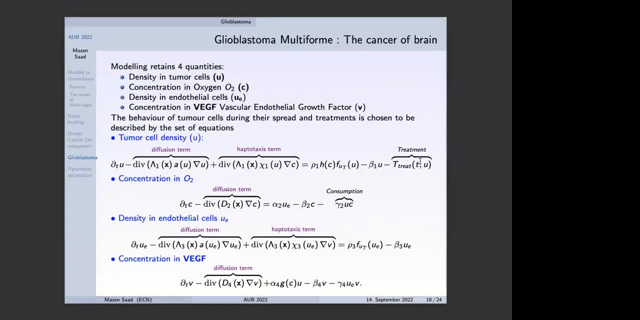 L infinity. okay, we. and the regularity of the solution is only A by gradient of U in L2, H1. okay, okay, it's not possible. if you want to more regularity, you have to derive this equation. so it's not possible. okay, but the minimum regularity. 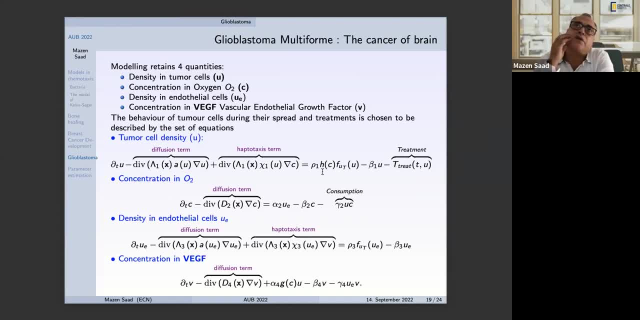 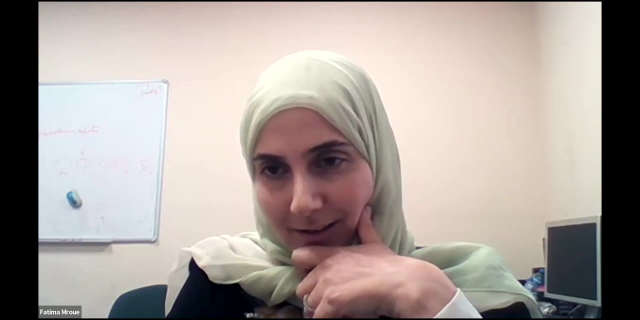 is enough for us to do a numerical solution and to show the existence. okay, this. this means that you have used semi-groups theory. result for second number in an affinity: yeah, okay, thank you. thank you for you. I see a question from professor. thank you for very for this very. 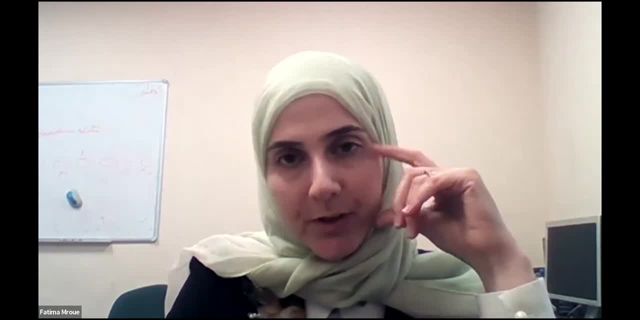 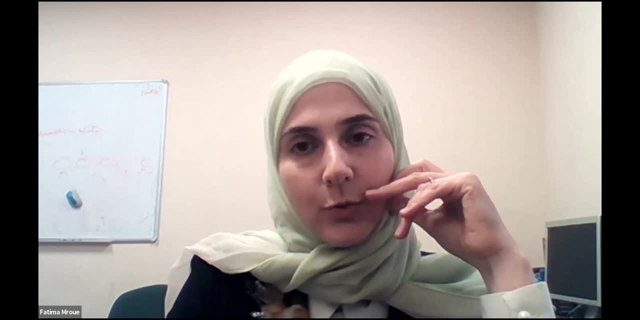 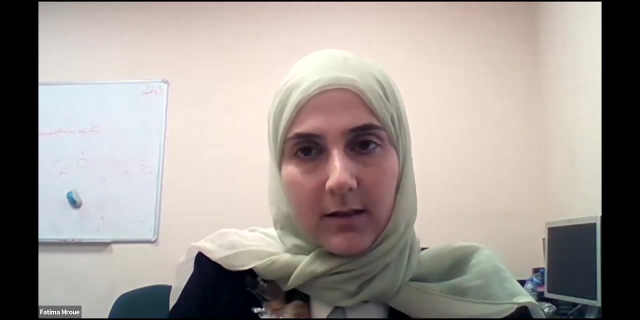 interesting talk regarding modeling of the brain tumor. are there any assessments for the coupling of mechanical stress and diffusion chemotaxis on tumor development? so do you have any idea whether there are any assessments, any evaluation or possible coupling between mechanical stress and diffusion in this case? yeah, I think for brain 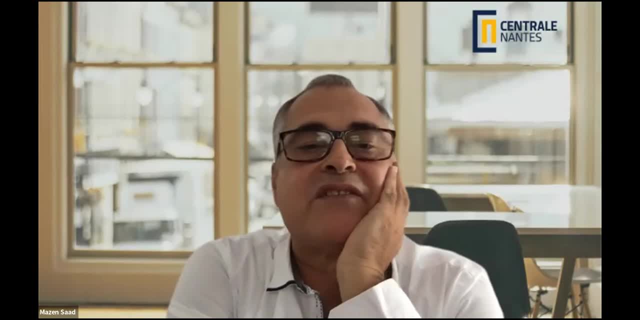 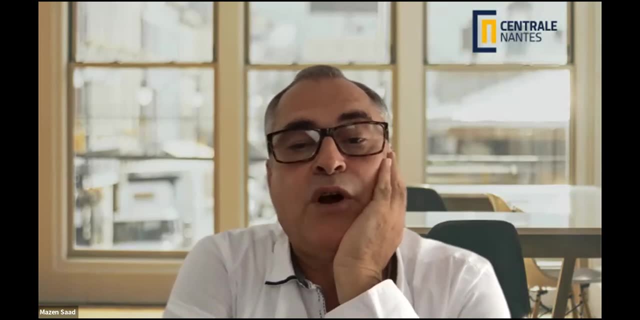 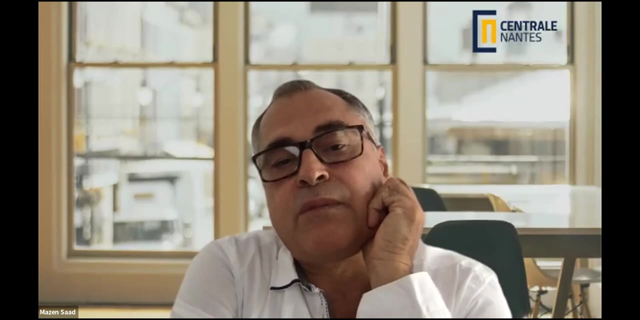 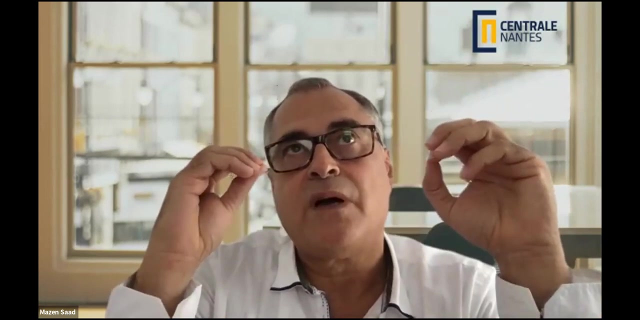 tumor, the mechanical stress is not. it's not important. but the mechanical stress is very, very important when, when you treat as a bone regeneration model because the fracture in general you have to to fix it to have the regeneration of the bone. but I think in brain tumor, no, there is. 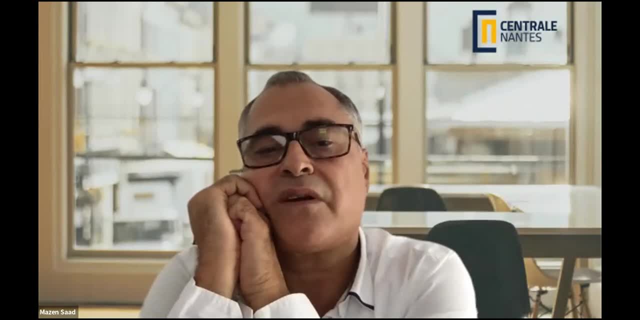 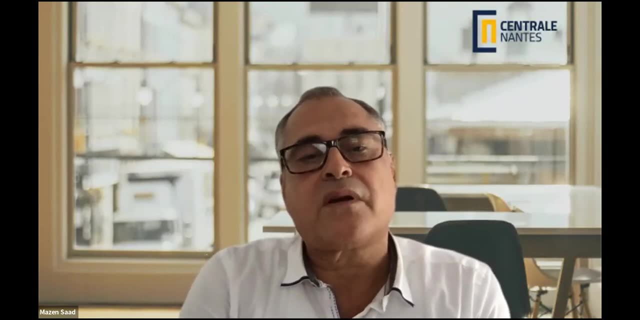 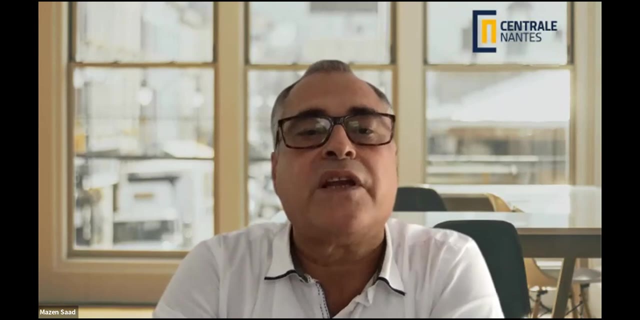 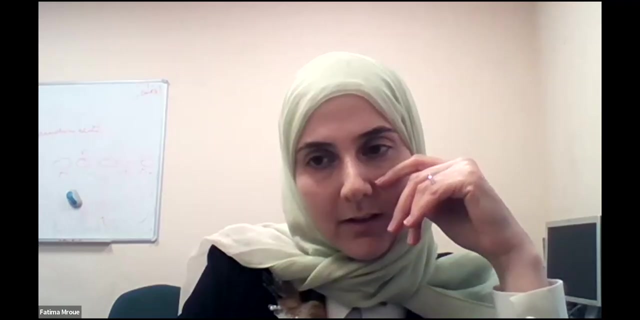 no, there is no constraint here, be because the tumor only is a, is a matter, is a white matter, okay, is there is no contract constant real content here. I think so that probably there is, I don't know, probably there is a possibility for some kind of coupling of mechanical 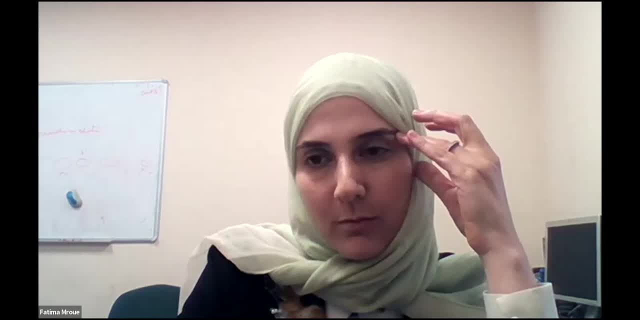 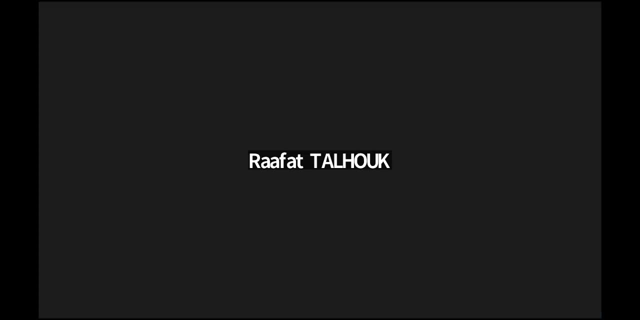 stress, probably because of the fluid, if you have an increase in the volume, I don't know. I think this is an interesting, interesting question. but coupling- coupling in fact it's always possible mathematically, but the problem is the study after if it's still possible and and easy or not, because 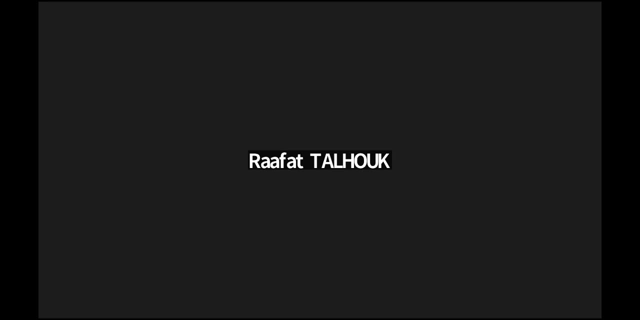 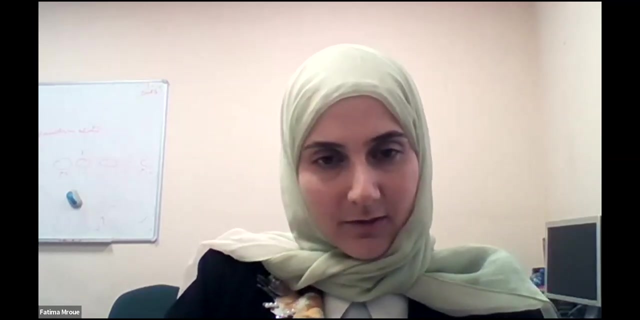 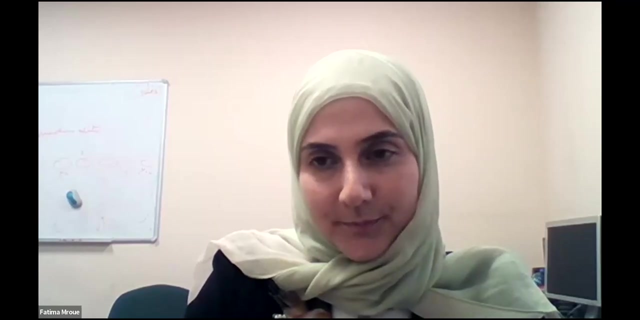 coupling with elasticity or stress equation maybe make appear more more, more, more complex problem and relevant problem. well, we have a question from professor Nassif. can you please understand? yes, I am unmuted, though. can you hear me? yes, yes, we can hear you. okay, good thanks. thank you, professor Saad, it's. 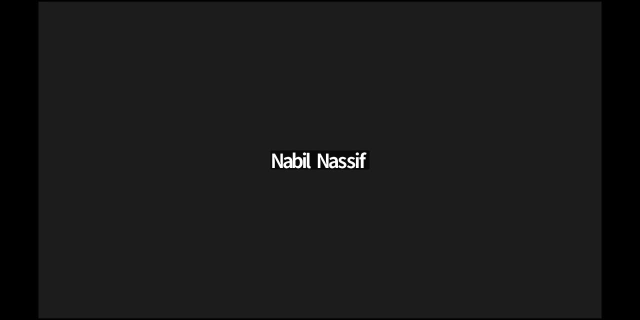 very interesting lecture I have. I couldn't really have see all your slides because I have a lot of had problems with sharing, with reading your, with reading your slides, but I read the first one and I'm I am. so you have essentially a system of two with two. 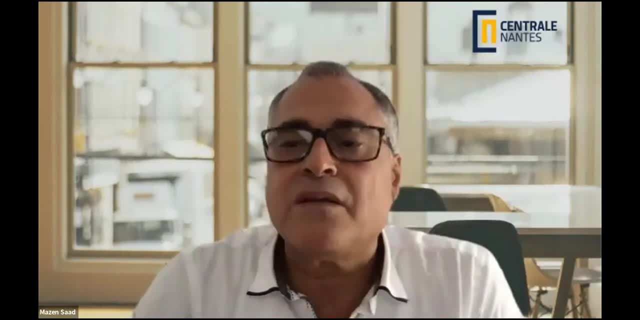 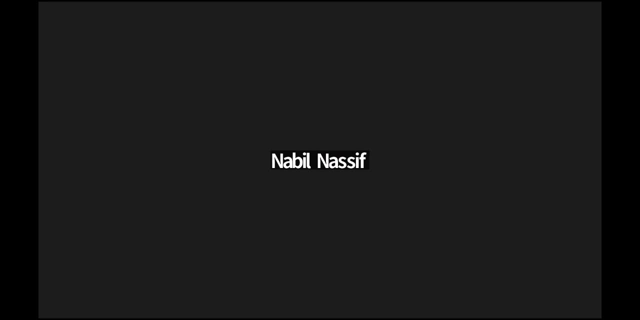 variables which are u and c. right, this is yeah, and and the involvement of the of these, of these functions is through some sort of, some sort of elliptic operator. and yet it is. you have, you have like two, two, two, two parabolic equations, yeah good, which are not non-degenerate. 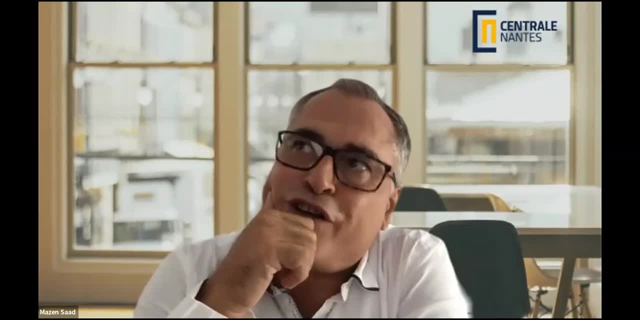 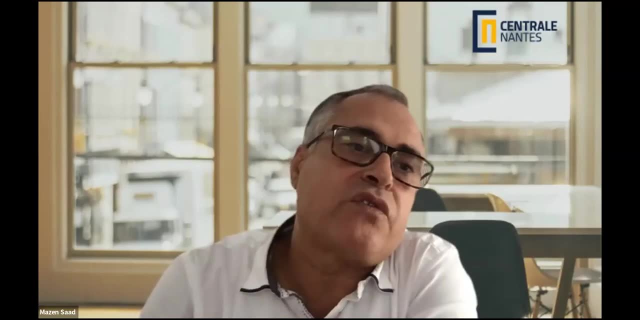 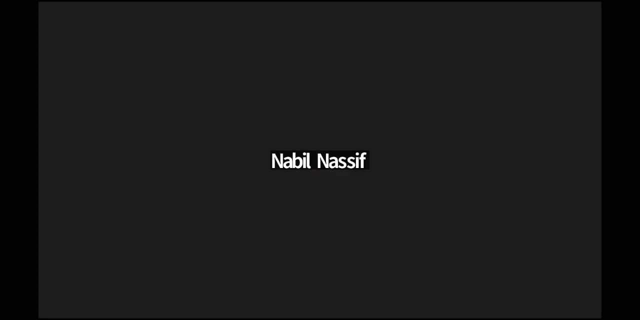 you see, that's right. no, it is degenerate. they degenerate, I mean the coefficient can go to zero or no. the, the coefficient here vanishes at zero and one. ah, okay, so this, this, what deteriorates, the regularity then, yeah, so for the gravity, and it is also 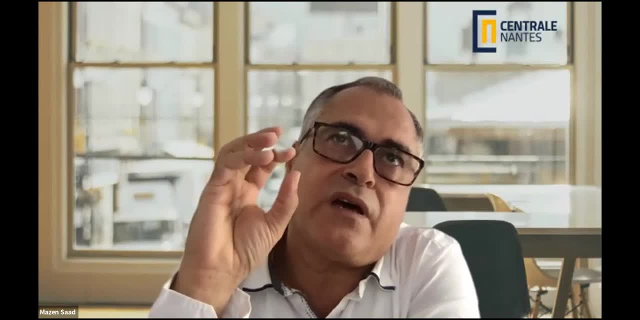 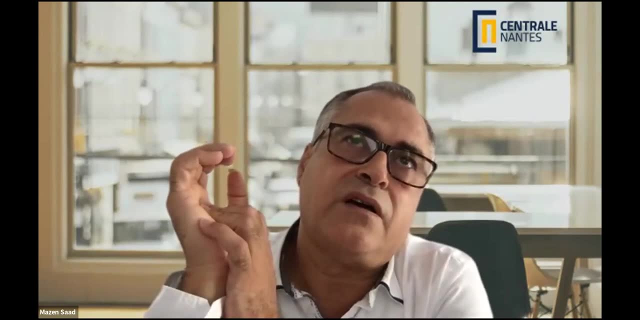 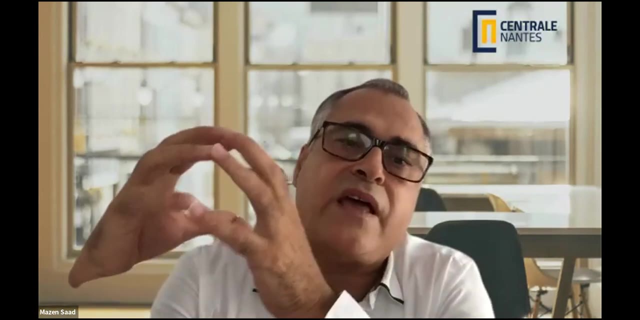 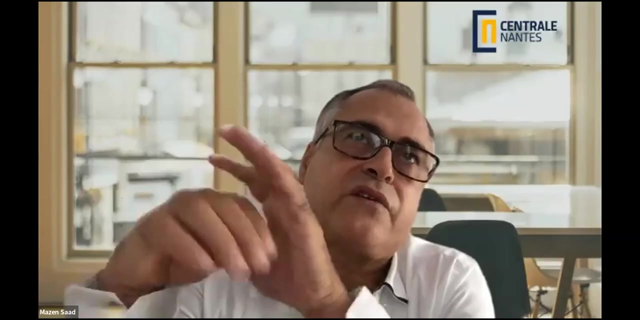 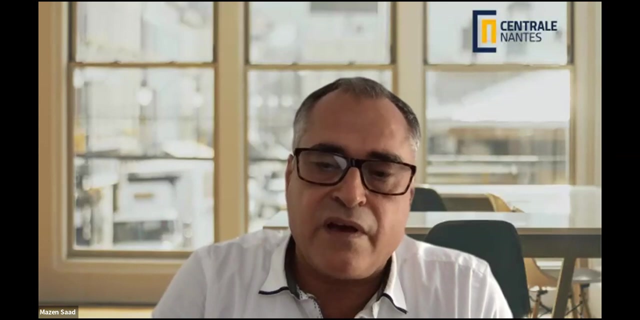 when the chemo attractant and vanish at one, it means that that the transport is vanished when the density of the tumor is maximum. we consider in the area here it is the we say here is a volume feeling effect, because if the, the volume is, comedy complete. 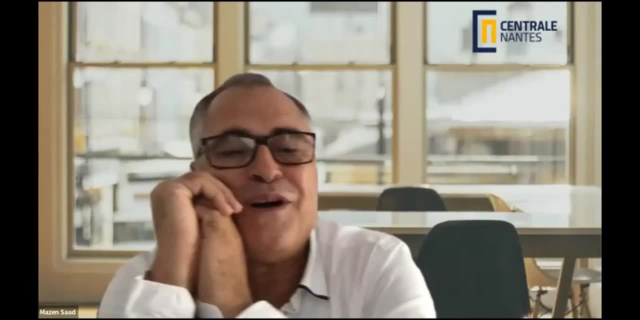 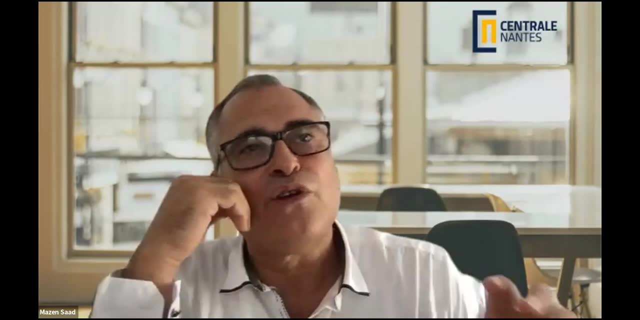 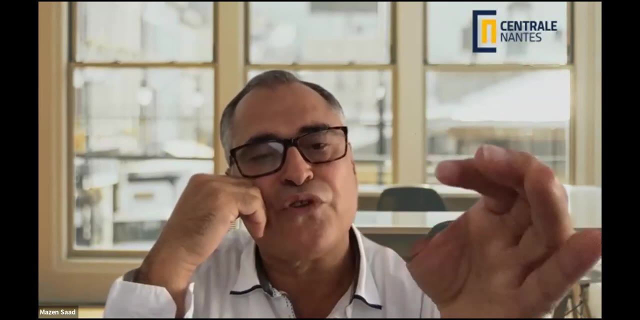 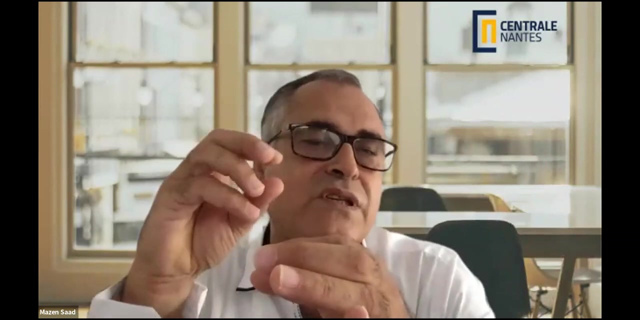 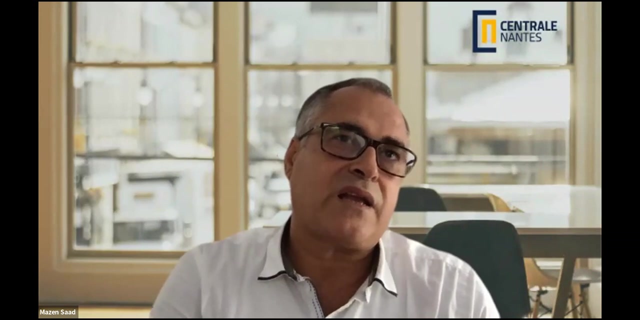 speaking french. ah, on the volume effects, the function suppose maximal, but after the zone time, in fact, the terms of diffusion, the coefficient of the function of division is also the function of sensitivity. so it's for that the tumor arrives, it is attracted, it is maximum, it will not move. 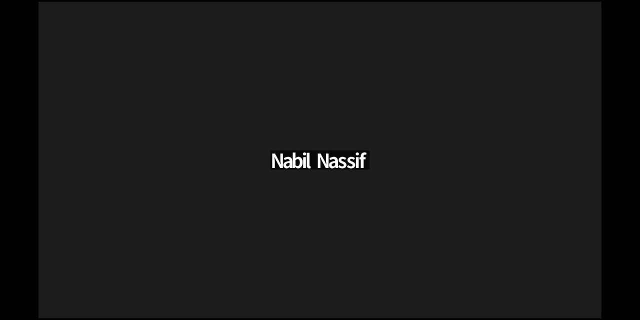 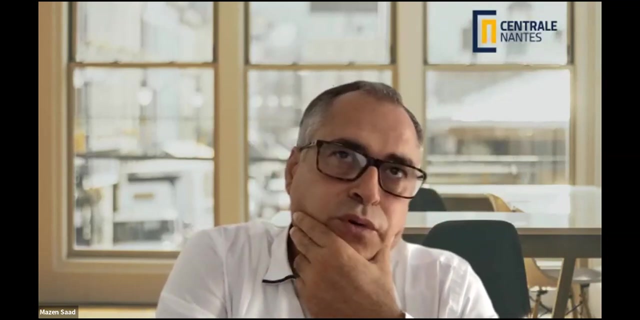 after it will move only by diffusion and the so. so there are phenomena of singularity. so, on the edges after uh, if we take a look at the function u, which depends only on u, we can consider that the solutions often the solutions and they explode in time finished. 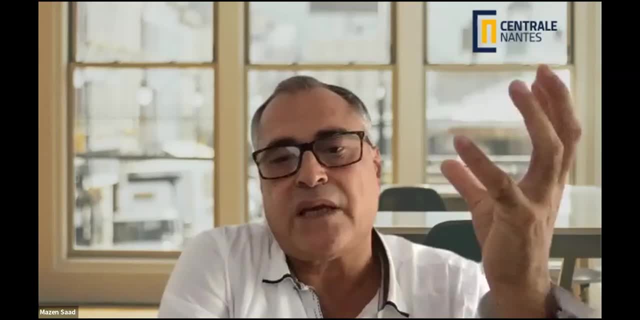 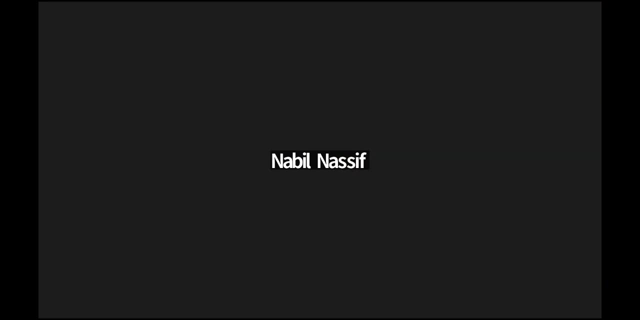 that is to say because this term, in fact it continues to attract the cells and therefore it will tend towards infinity. so we lose the principle of maximum. and now, how do we do it numerically, if there are phenomena of explosion, how do we control? uh, how do we do? 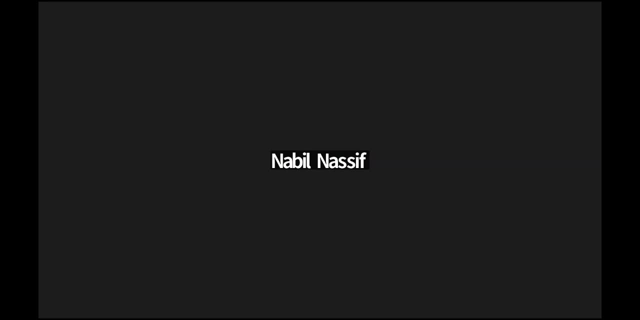 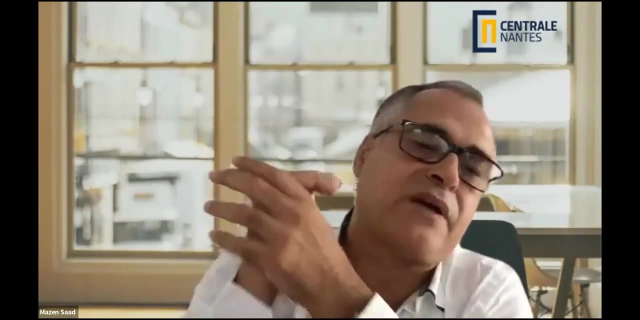 how can we do it? we regularize in general around and numerically we are obliged to change at a certain moment the solution: okay, the cells, still numerically it will be a maximum and we consider from that it is, ie, the solution to the explosion. 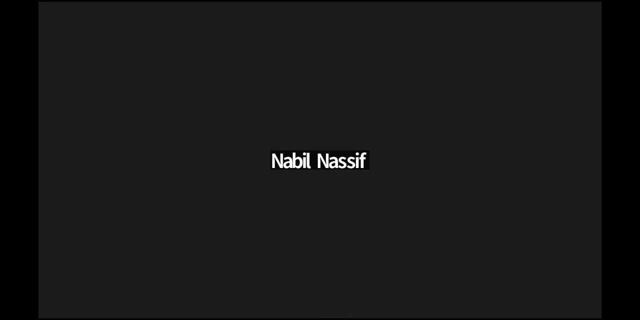 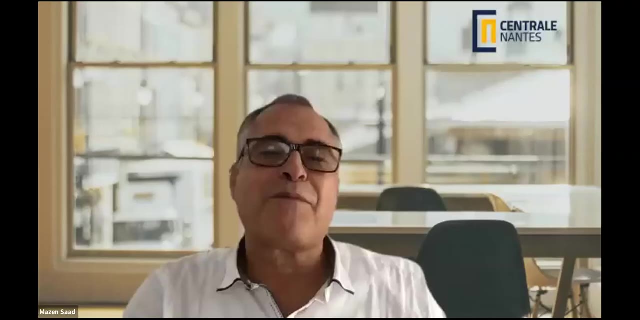 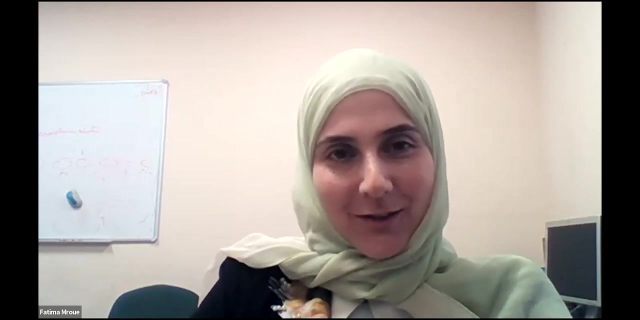 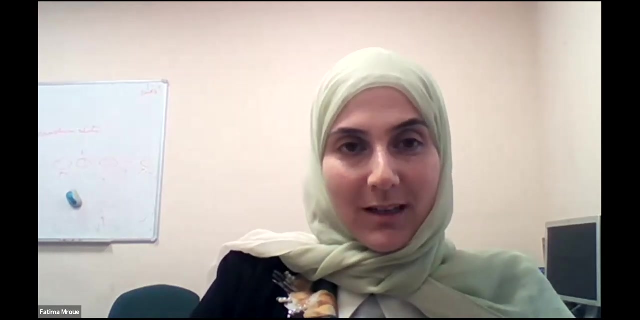 very well, thank you, thank you, thank you. any other questions from the audience? arabic now. well, um, just take a general question. i don't want to go into mathematics at the end. uh, do you have? well, we, we saw that you're you're exposing many mathematical. 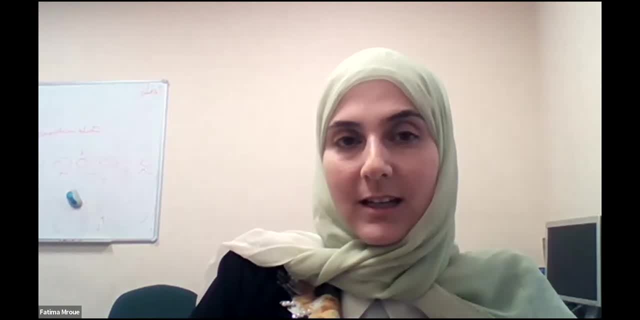 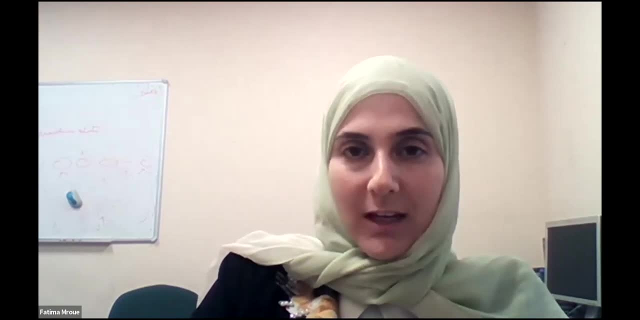 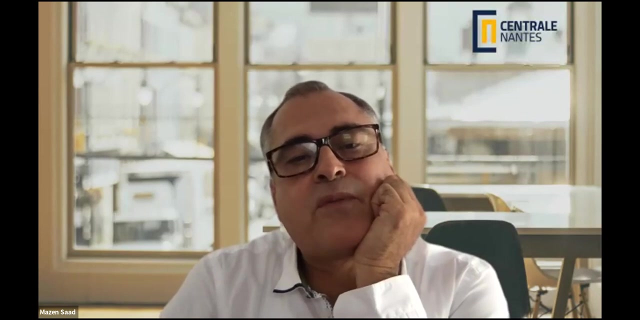 models. what is the the use of? is there a feedback from from medical doctors about your results? is there a usually a communication whenever you're doing such uh such a work? okay for uh, for the last one, uh in glioblastoma, because uh, uh, this work is in collaboration with a. 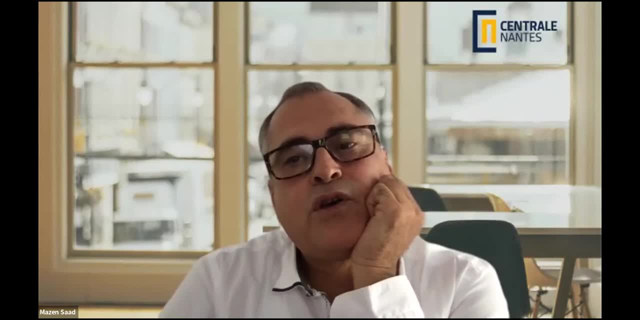 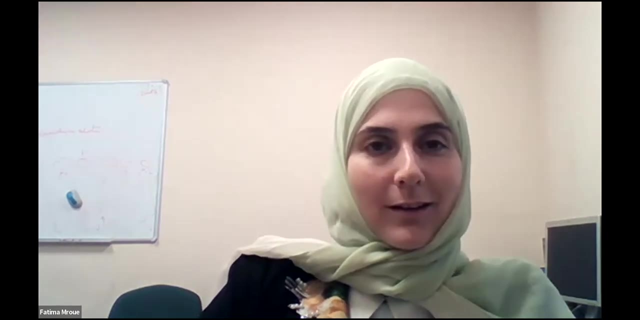 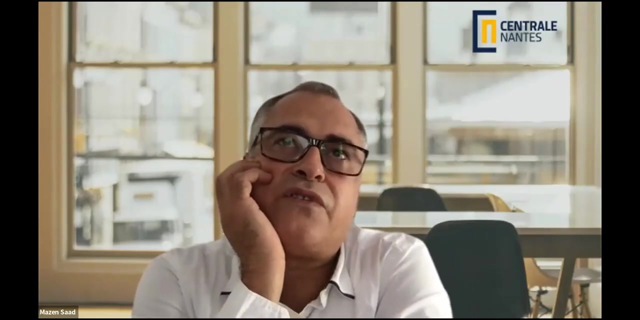 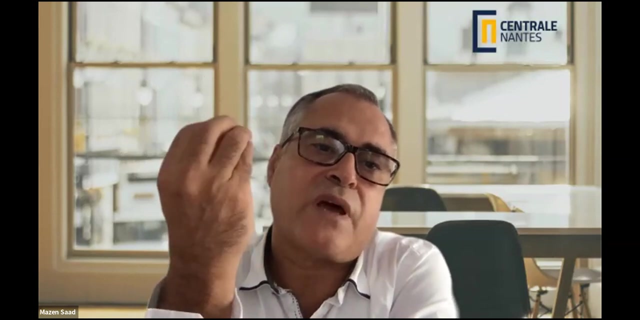 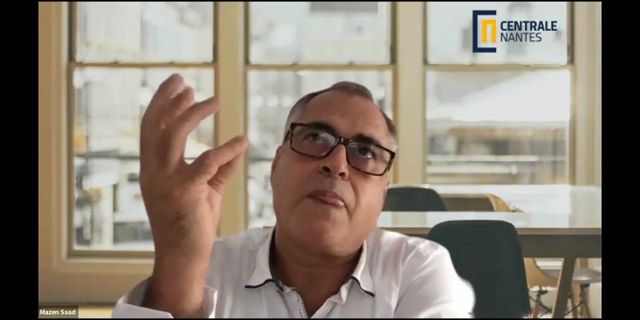 biologist which works here in the hospital and we discussed with with doctor to validate this problem. so there is always kind of uh, continuous communication between the modeling people and the and the medical, exactly biology in all these structures. Yeah, Our aim is to use MRI to adjust the parameter. If you have the good parameter for the patient because it's different, and if you have a good numerical simulation, we can after perhaps give the best treatment for the patient.